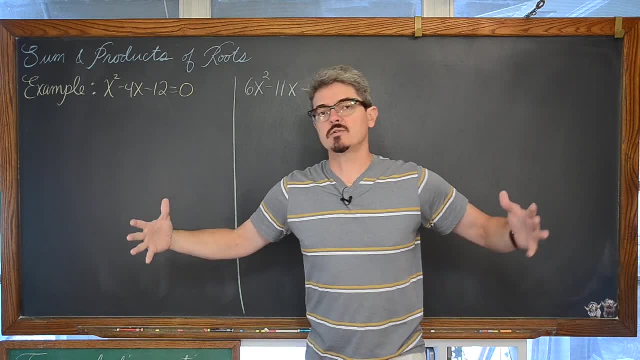 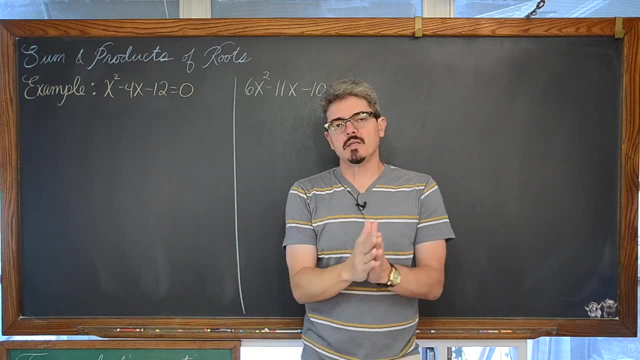 that we have had before. In an upcoming lesson we are going to extend this idea to not just the sum and product of roots of quadratics, but actually at the core concept that is, in this lesson it actually extends to all polynomials. So let's get started first by reviewing how 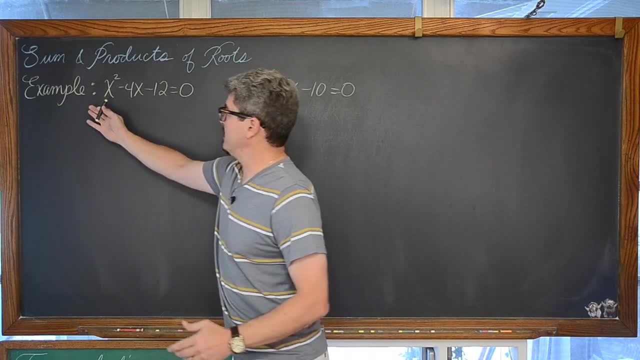 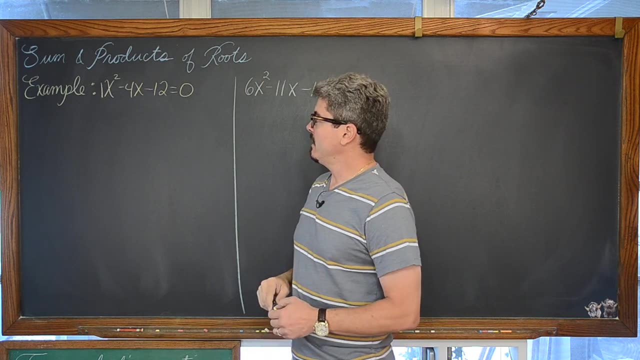 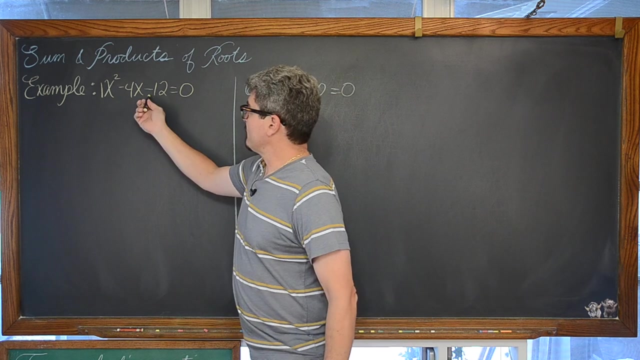 to factor. So we have here a quadratic with a leading coefficient of one. We have a constant which is negative, set equal to zero. We are going to factor this by simply looking for factors of our constant which is negative. twelve that add to the middle term Our factors of negative. 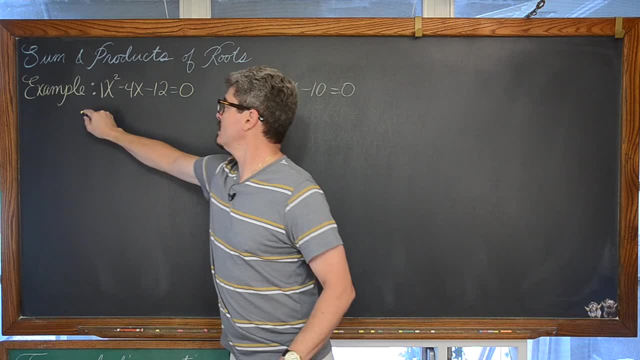 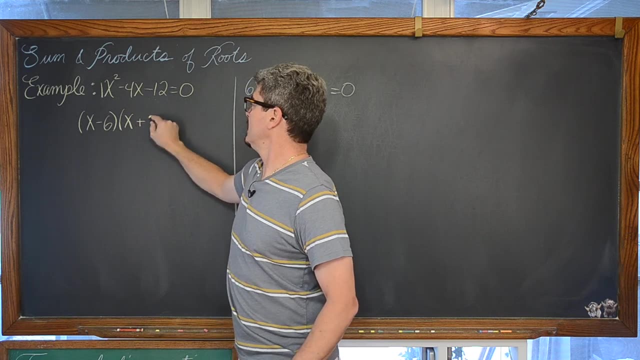 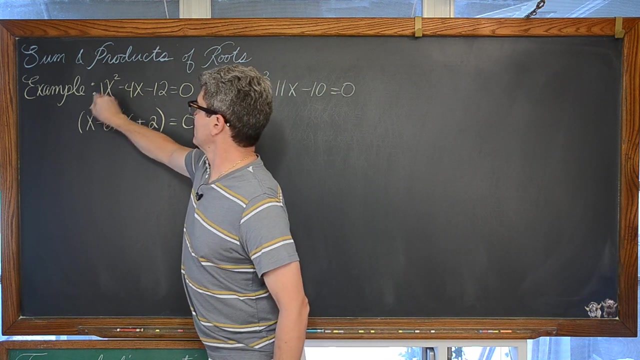 twelve that actually add to be negative, four are going to be x minus and so a factor of negative six. Then we have x and a factor of positive two. So we have our factors of our first term going in the first two blanks of our two factors. 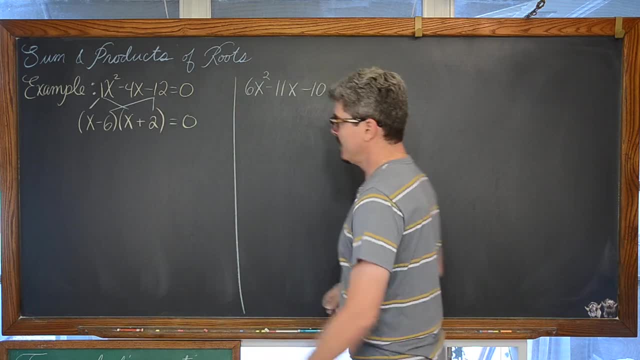 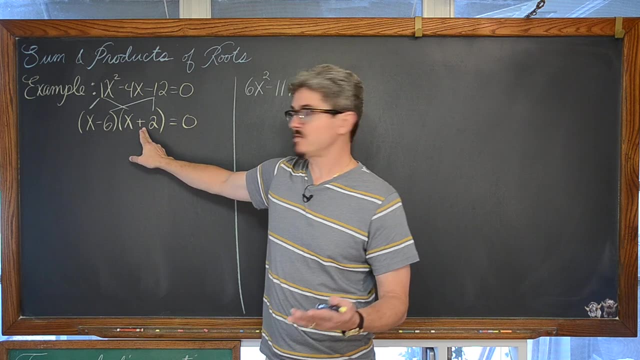 here The factors of our constant going in the last two blanks. If we want to double check this, we are just going to simply distribute this back together. We have: x times x is x squared. x times positive. two is two x Negative. six times x is negative. six x, Of course, negative. 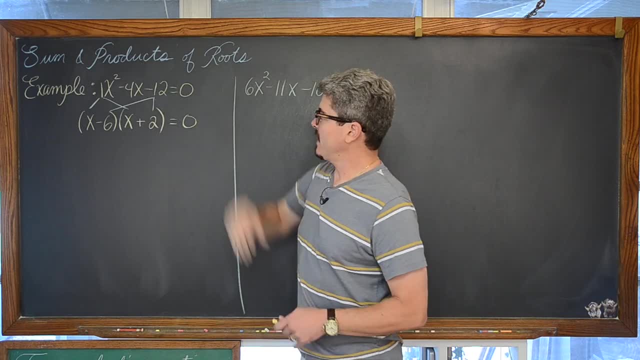 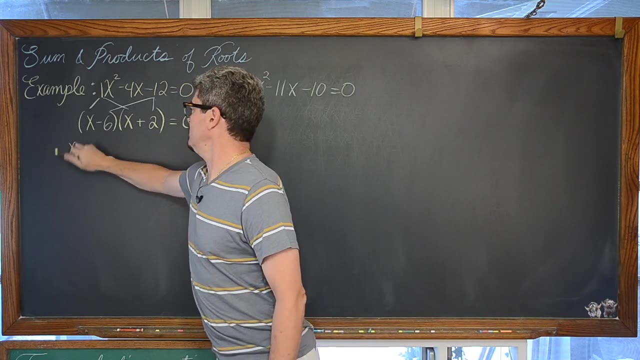 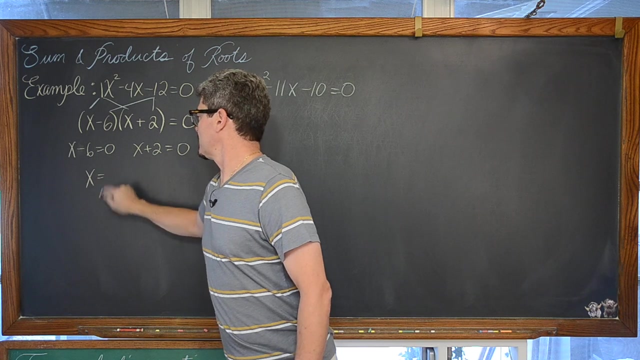 six, x plus two, x is equal to negative four. We have negative six times two is negative twelve. Of course, we are going to set each of those, So we are going to set each of the these factors now equal to zero. We end up with: x is equal to six and x is equal to negative. 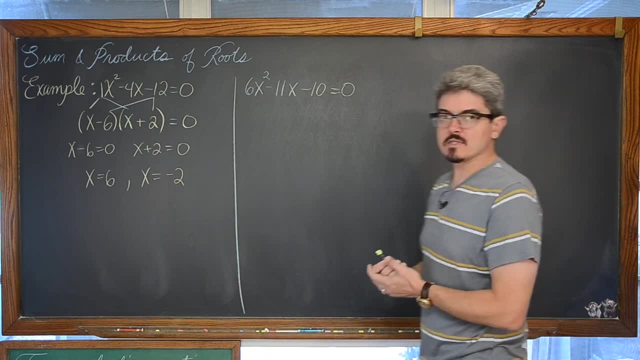 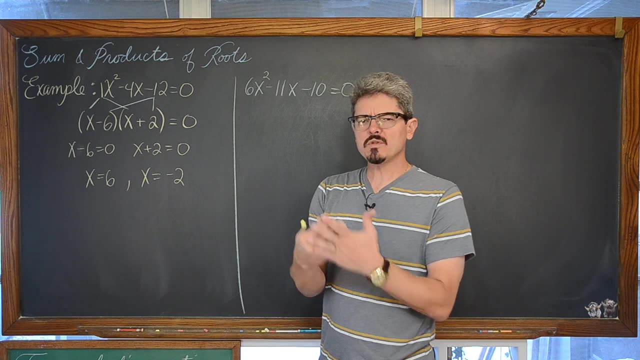 two. Now, the whole point of this lesson is to not just talk about solving quadratics and not even just necessarily looking at the core roots. but what do they add up to? Well, the sum of six and negative two is equal to zero. So we have x plus x squared plus. 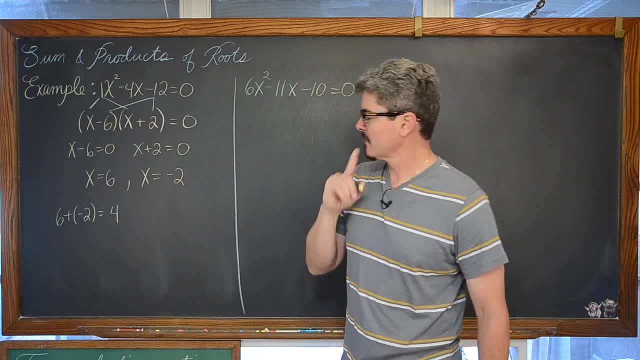 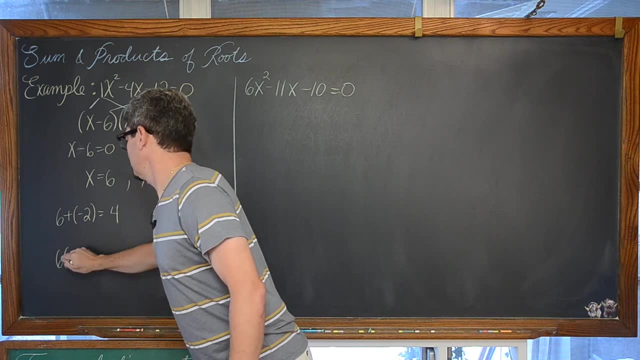 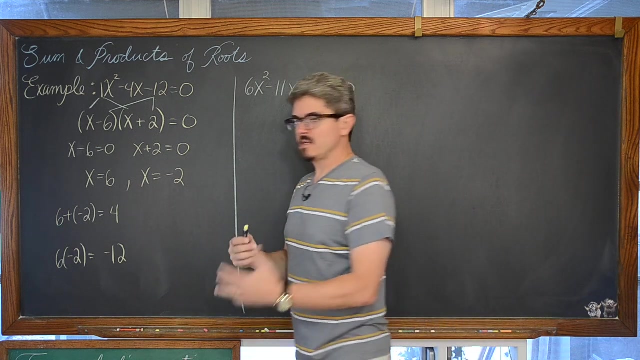 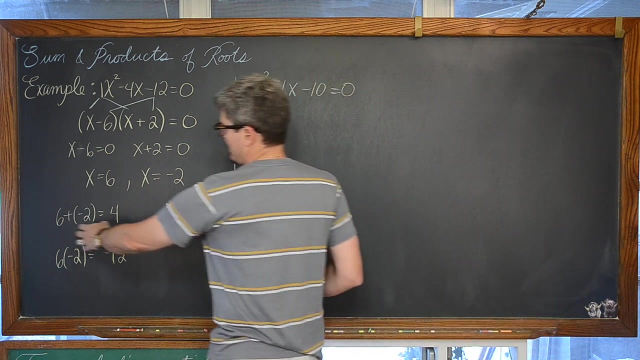 two is equal to four, The product of six and our other root of negative two is equal to negative twelve. Well, especially since our leading coefficient is one here, or basically our coefficient of a in our quadratic equation, we have that the sum of our two roots is coming. 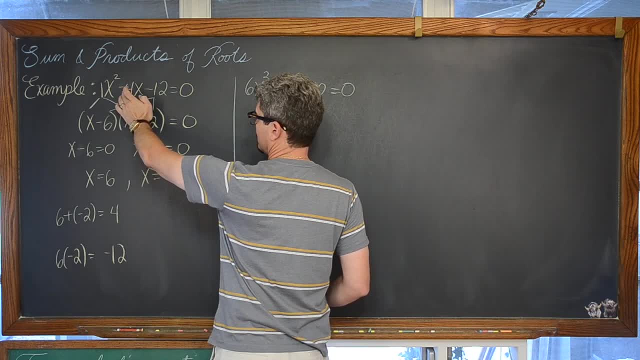 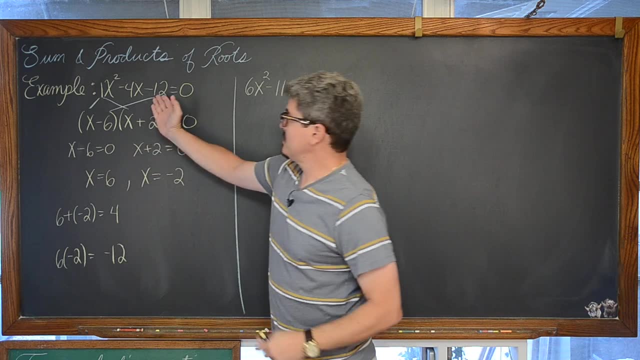 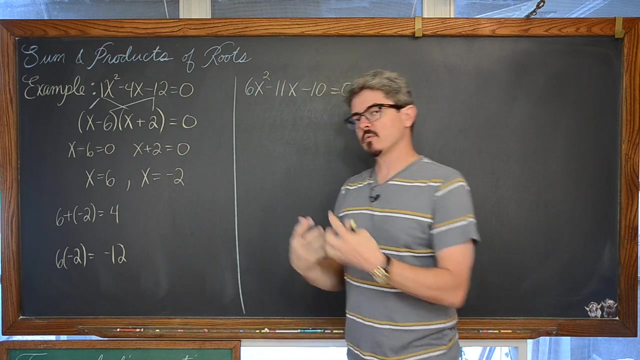 up to not the middle coefficient here, But it seems like it is just the opposite. The product of our two roots is equal to our constant, But with our leading coefficient equal to one. we are not getting the complete picture here about the relationship of the sum and. 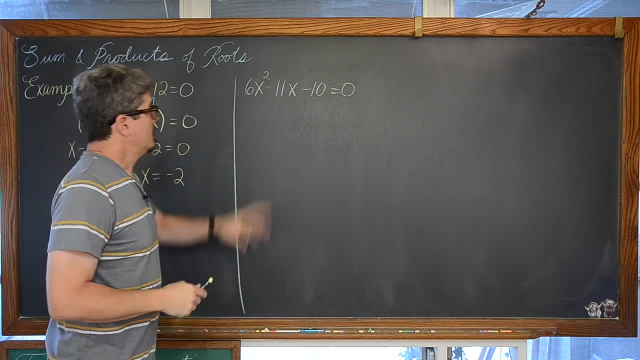 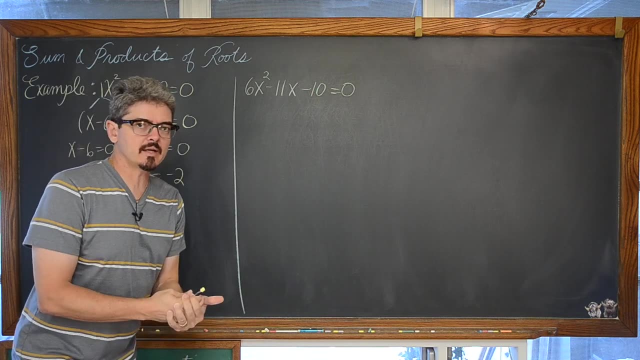 the product of our roots for a quadratic. So let's take a look at this example Now. with this example, we have a leading coefficient which is not equal to one. So without being forced to do trial and error or just a little graphical trick that sometimes we see in the 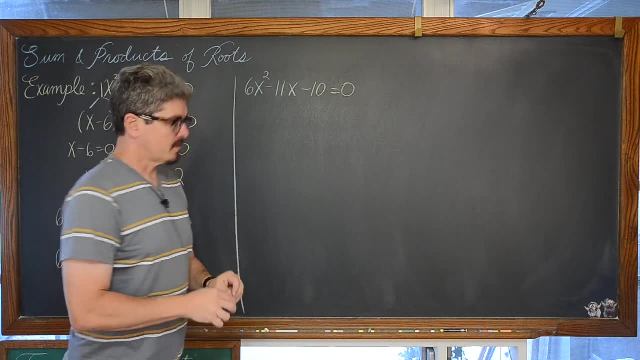 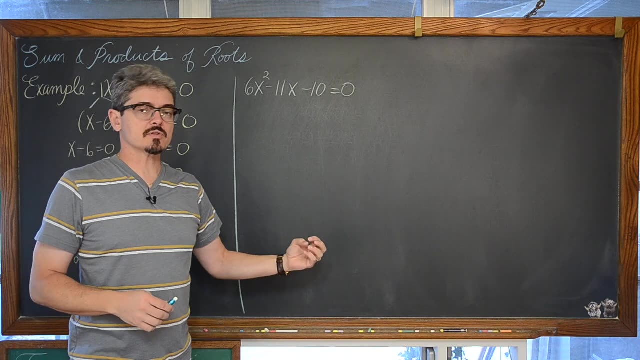 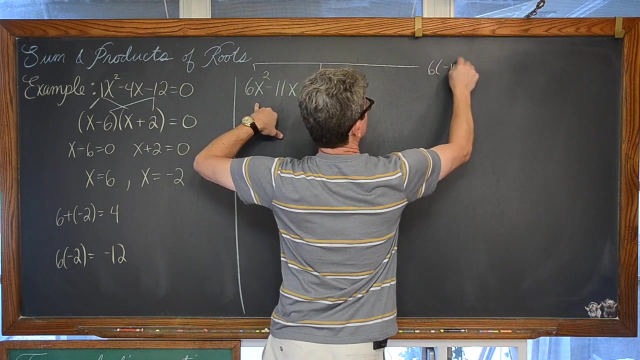 algebra books. now we are going to go through the process of reviewing. factoring by grouping. that is going to allow us to solve this quadratic without trial and error. That is going to be taking our leading coefficient and our constant. We are going to multiply those together and 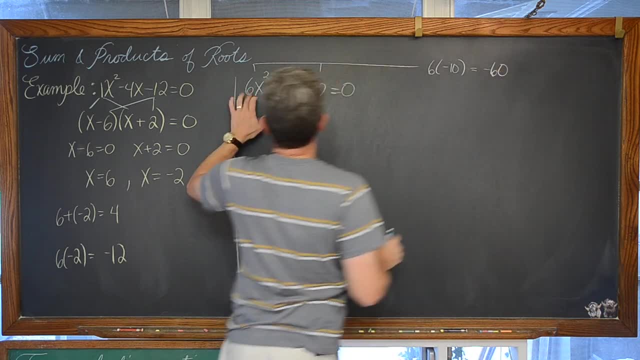 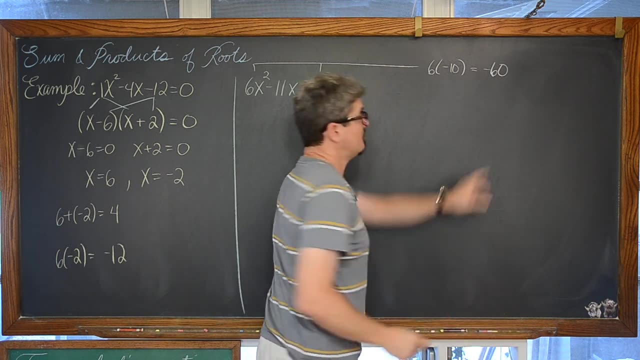 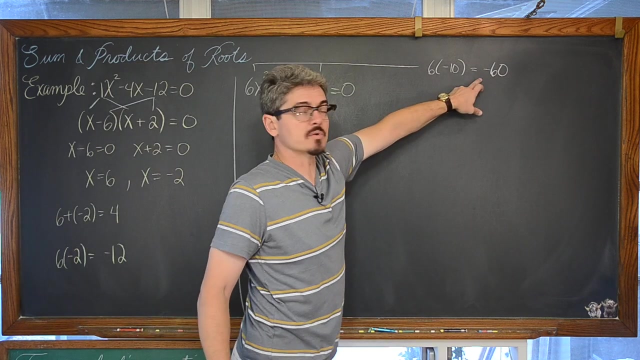 get some kind of product. Well, six times negative ten is negative sixty. Now we are going to be looking for factors of this negative sixty, One of the factors of the negative sixty 60 that add to the middle term of negative 11.. We do have a product which is negative. 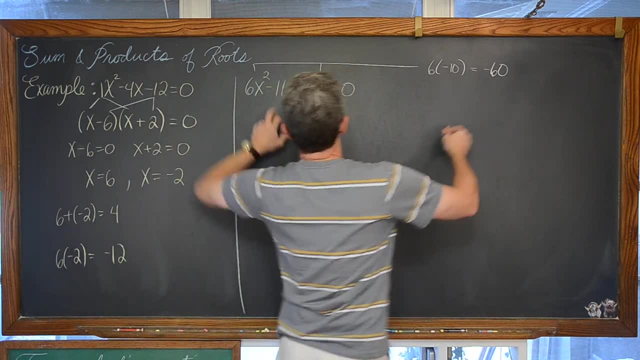 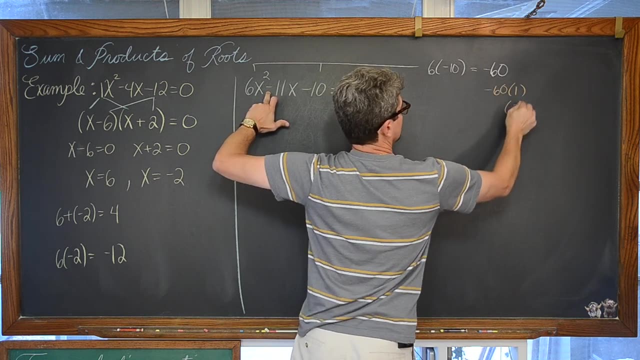 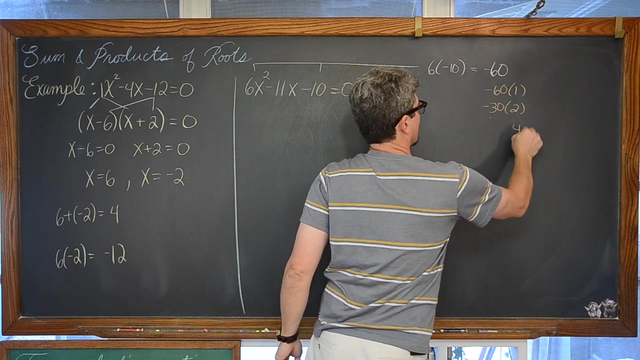 so we are going to have to use factors, of course, that have different signs. We have something like negative 60 times 1.. We have 2 times negative 30. That adds up to be negative 28,- nowhere near negative 11. But we could use 4 and multiply that by negative 15.. Now 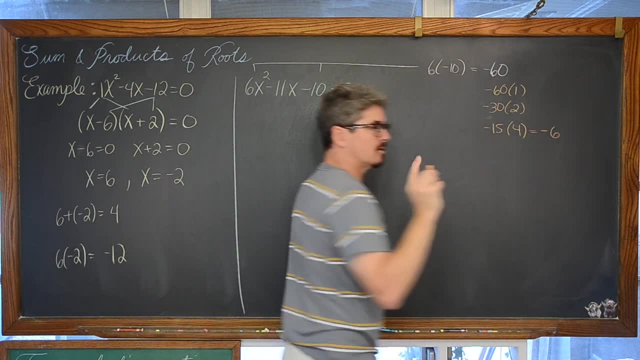 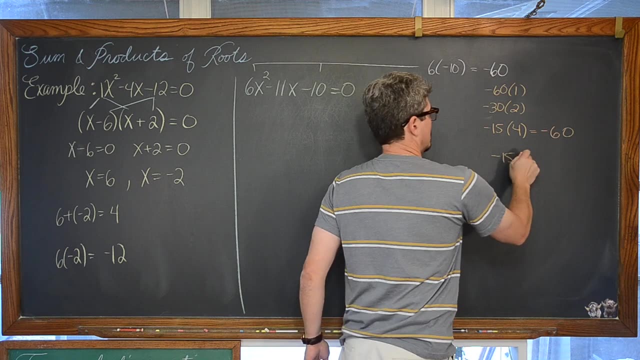 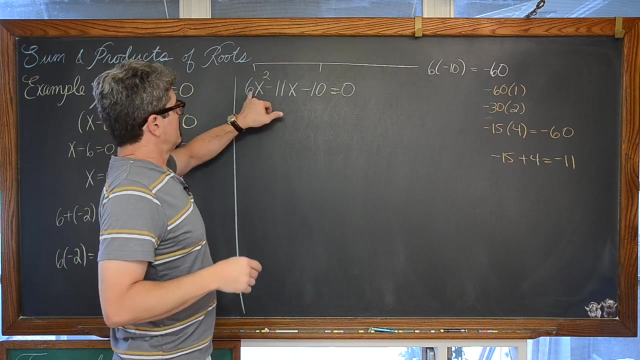 4 times negative 15 is equal to the negative 60, but the real magic here is that negative 15 plus 4 is equal to negative 11.. That is matching here our middle term With the product, the factors of our product that we got by taking the leading coefficient and the constant. 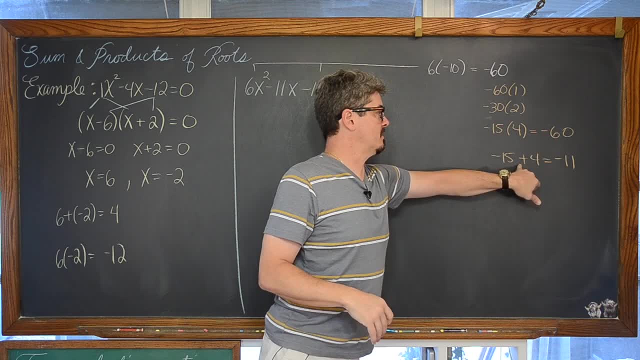 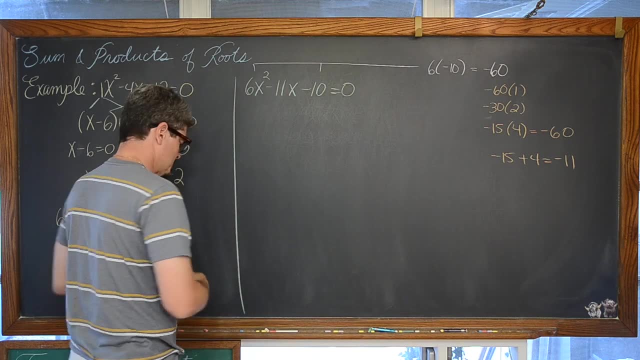 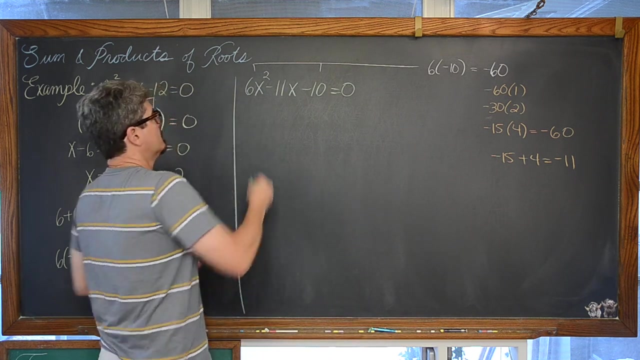 and multiplying it together, the fact that this special set of factors of negative 60 also, Let's also add to the middle term, or basically coefficient, which is negative 11. We are going to use that to rewrite our trinomial as a four term polynomial. We have 6x squared. 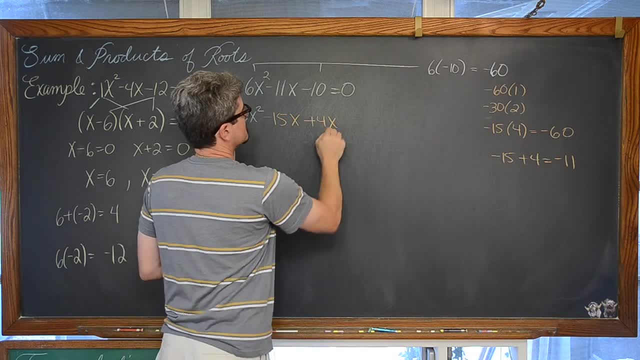 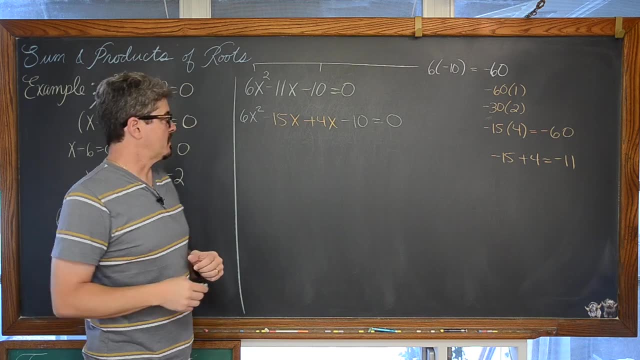 We have minus 15x, plus 4x, We have a. minus 10 is equal to 0.. Now that we have our trinomial written as a four term polynomial, we can factor by grouping, As long as this process over here in orange has worked out. 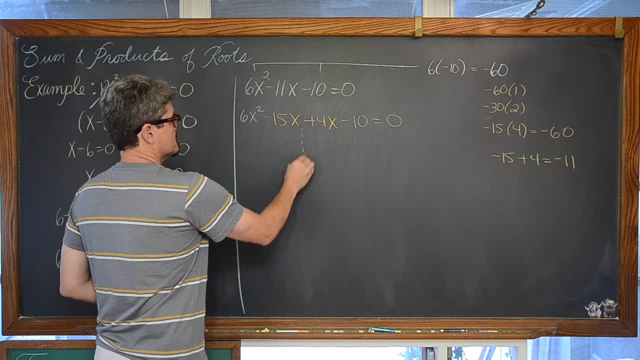 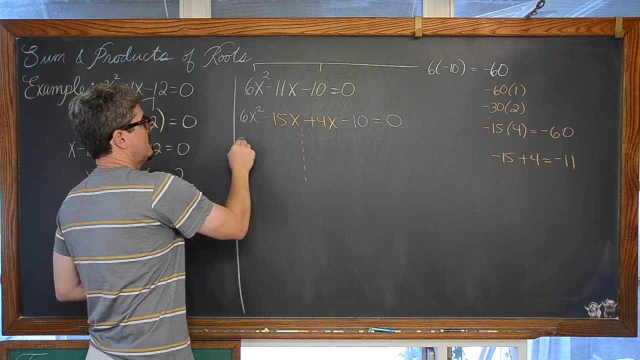 Now let's do the next step. We have done this properly. We are going to look at the first two terms separately and realize that we can take out a factor of three and x. So we are going to have a 3x. 6 x squared divided by 3x is equal to 2x. We have 15x divided. 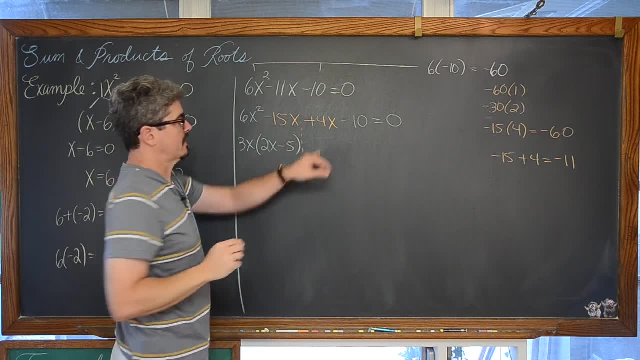 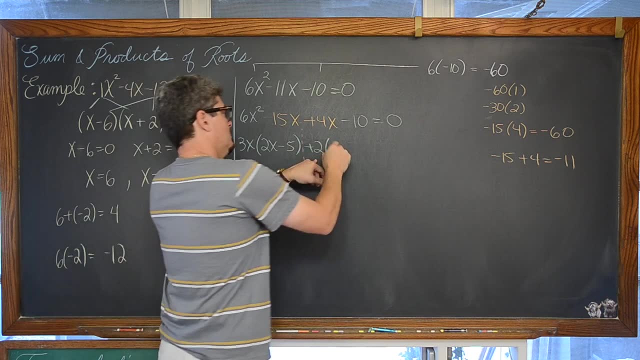 by 3, which is going to give us negative 5.. Now our last two terms. here we can factor out a positive 2. We have a plus 2. 4 divided by 2 is equal to 2. So we have 2x Negative. 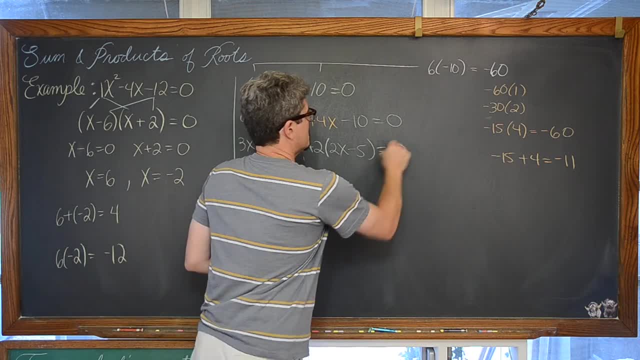 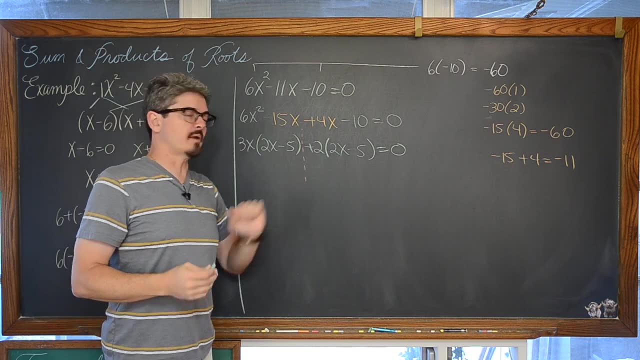 10 divided by 2 is negative. 5 equals 0. And we have this one plus sign separating these two big terms. Basically, there is a term on the left and the right hand side of my red dotted line. Each of these two terms have a common factor of 2x minus 5.. So if we take 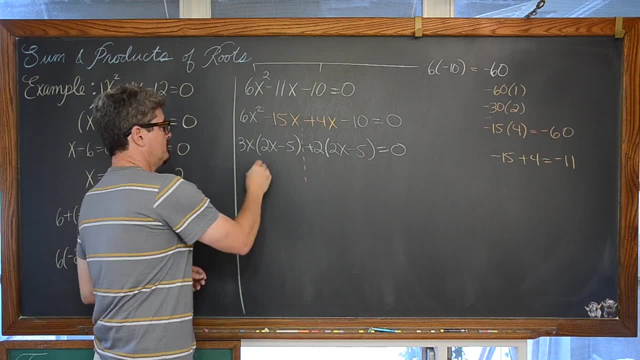 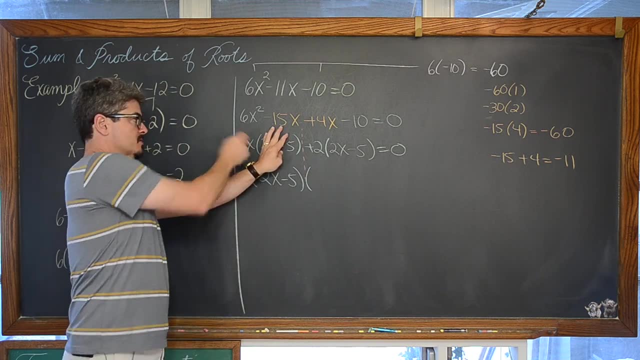 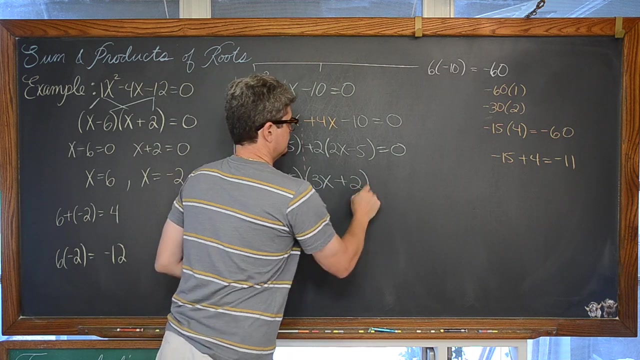 that common factor of 2x minus 5 and factor that out. well, out of our first term, if we take out that 2x minus 5, we are just left with a 3x. And for our second term, if we take out that 2x minus 5, we are left with a 2.. And now we have this quadratic equation: degree. 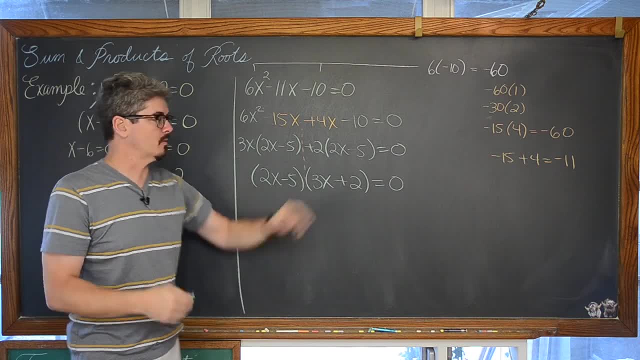 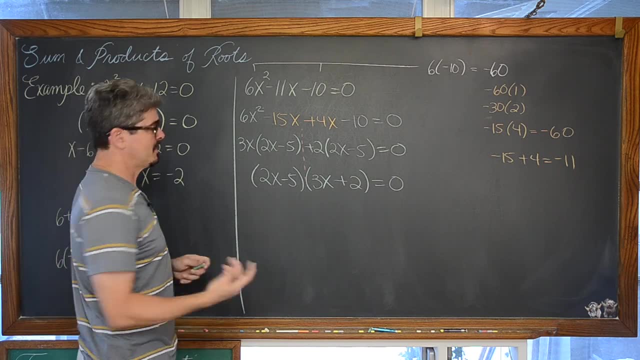 of 2 with a leading coefficient other than 1, we have been able to factor it without having to do any kind of trial and error. that I was taught back when I was in high school many, many years ago. You can see all the gray hair. If you multiply this back together to 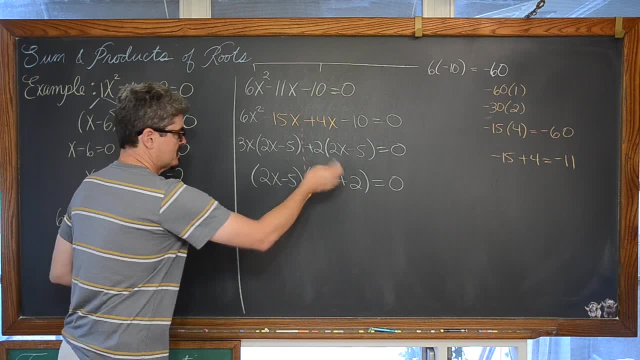 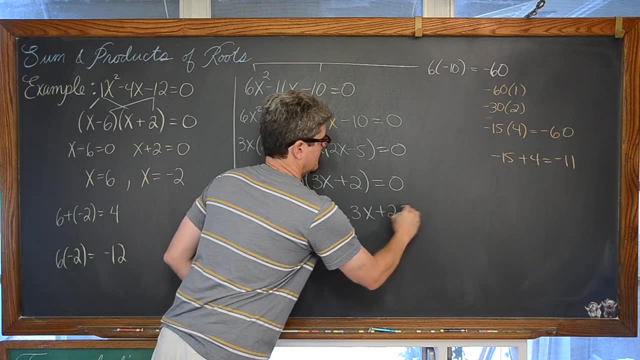 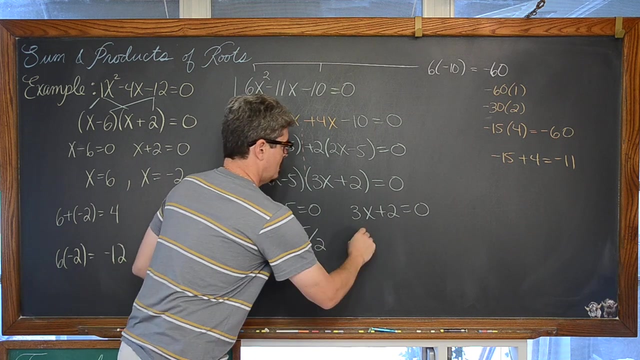 double check it, you will have our original Trinomial. Of course, now we are going to set each of these equal to 0 and finish solving Subtract both sidesor. add both sides by 5 and divide by 2.. And here we are going to. 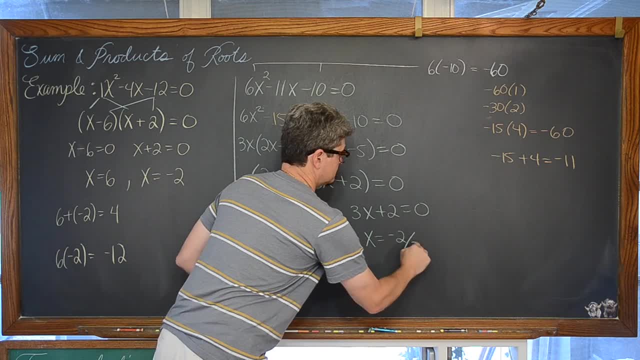 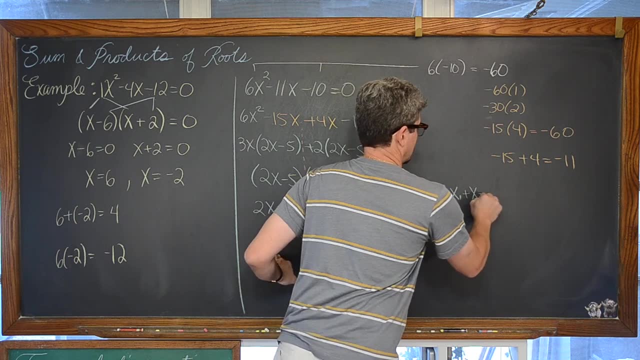 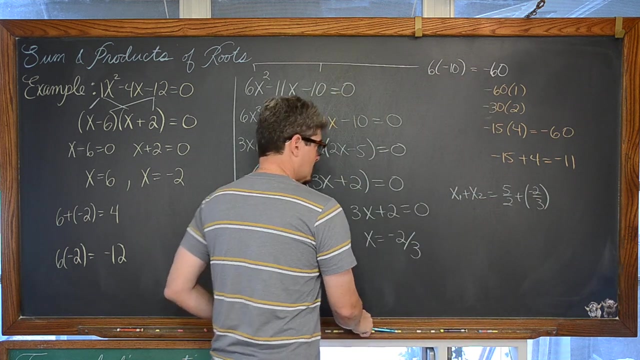 subtract by 2 and divide by 3.. And we have these two roots here. So we are going to look at the sum. So we have 5 halves plus negative 2 thirds. We are going to need to find some common denominators, So we are going. 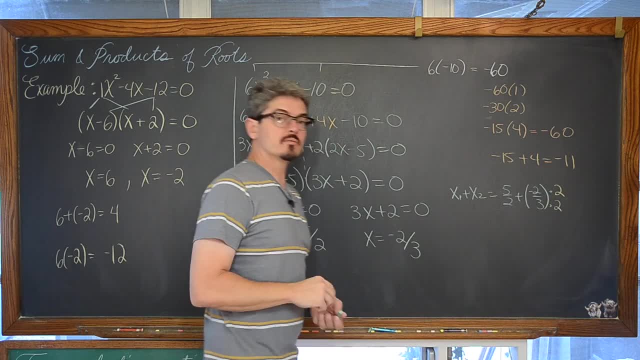 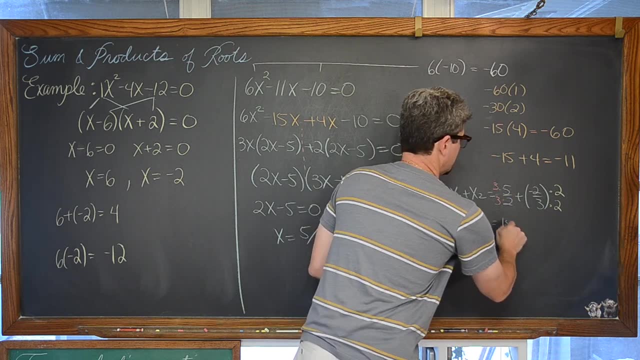 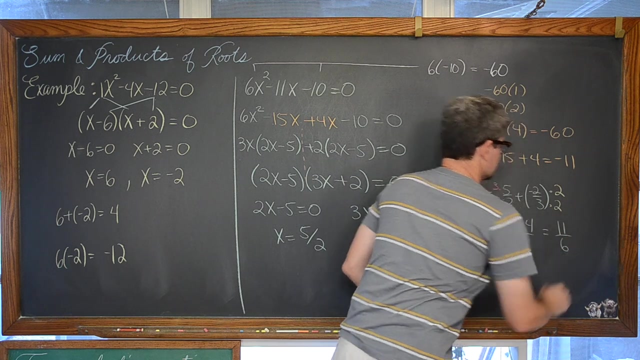 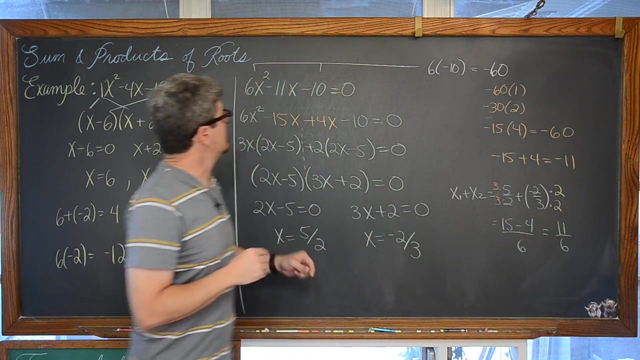 to multiply this second fraction by 2 in the numerator and denominator And this first fraction by 3, giving us 15 minus 4 over the common denominator of 6. And we have 11 over 6.. Now the sum of our two roots. 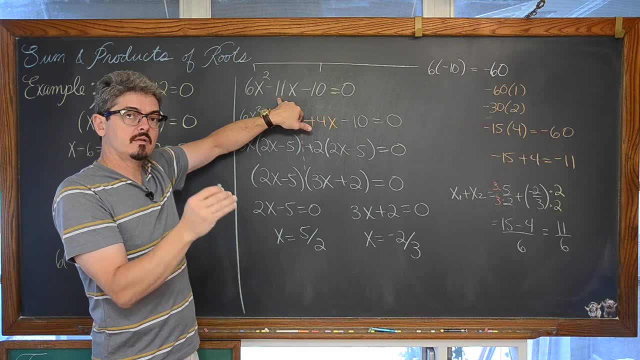 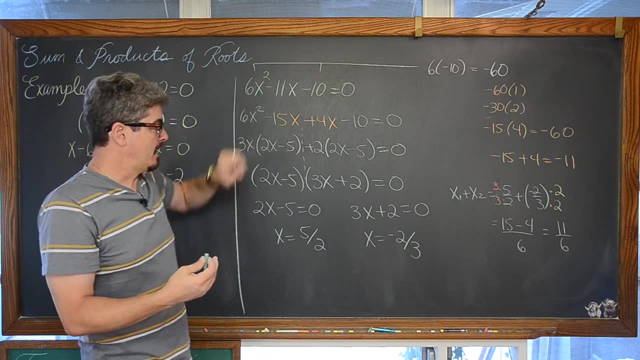 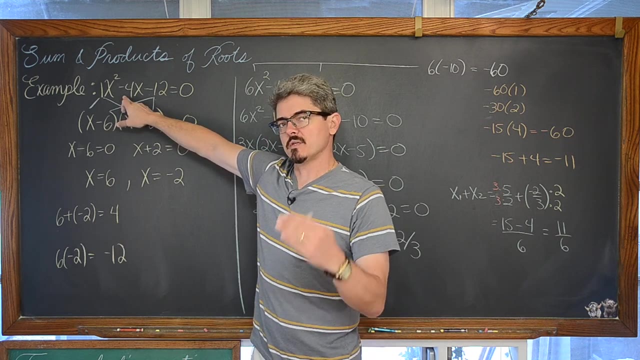 see we have 11 almost Negative. 11 is our coefficient of b, And we have 6, which is our coefficient of a, And over here we had, the sum of our two roots gave us 4.. Well, it looked like we were just looking at the opposite of the middle term, But that is just simply. 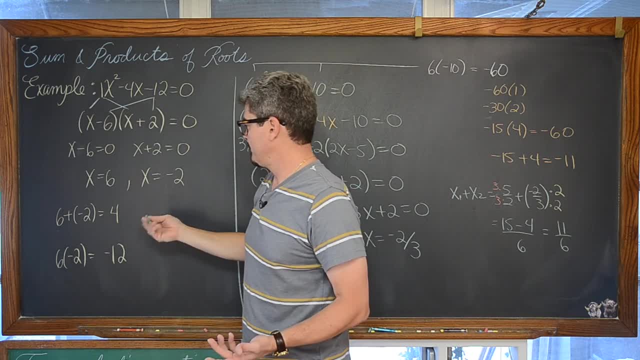 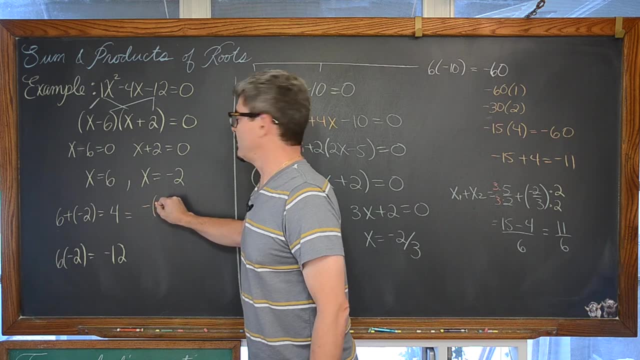 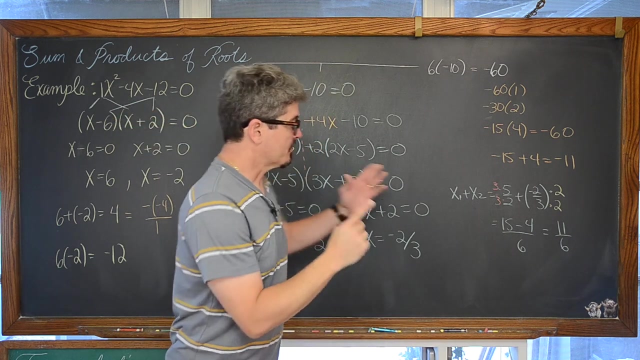 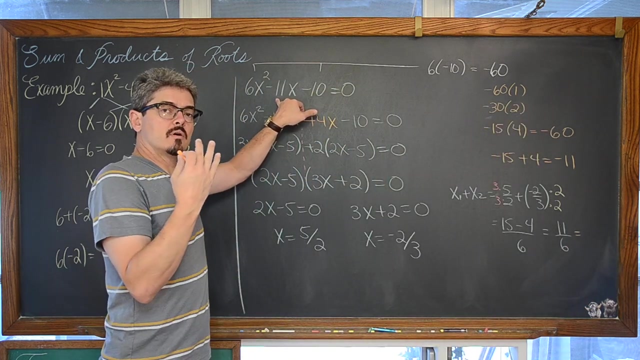 because our leading coefficient is 1.. So really, this isthis: 4 is equivalent to taking the opposite of our middle coefficient and then dividing that by our leading coefficient of 1.. Or, over here, our 11 over 6 is the equivalent of doing the opposite of ouror taking the opposite. 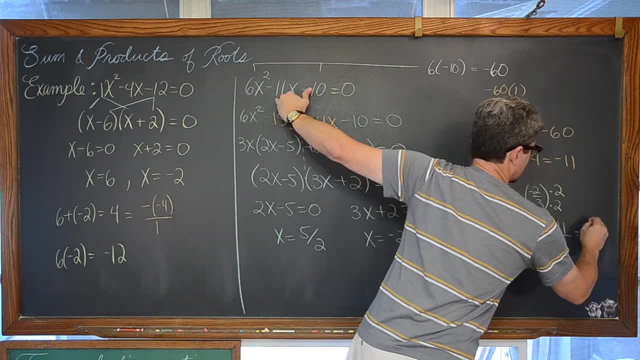 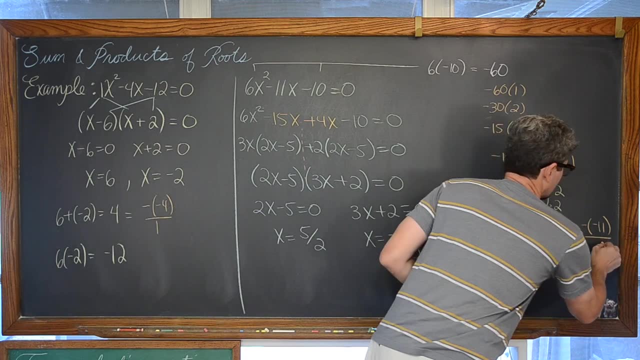 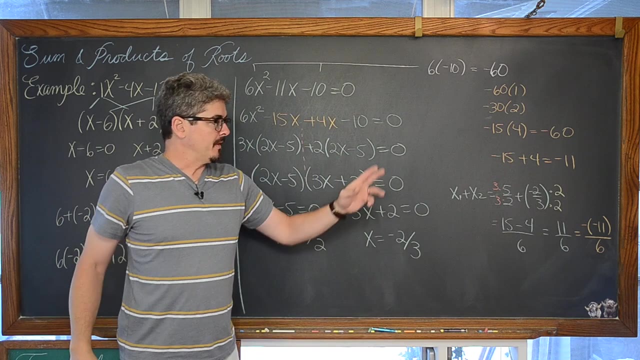 of our middle coefficient b and dividing it by our leading coefficient, or coefficient of a Sowhoops. I am thinking about what I am about to show you. I am going to show you here as a sort of summary statement. The sum of the two roots of a quadratic is equal. 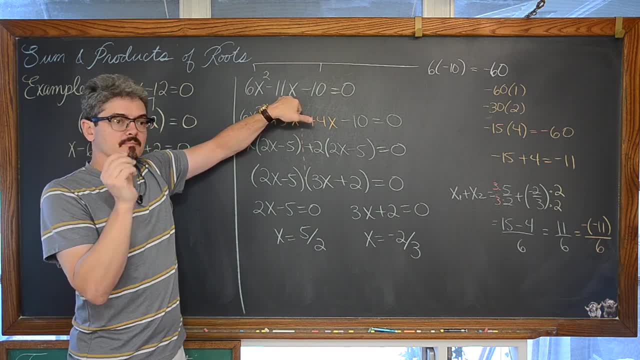 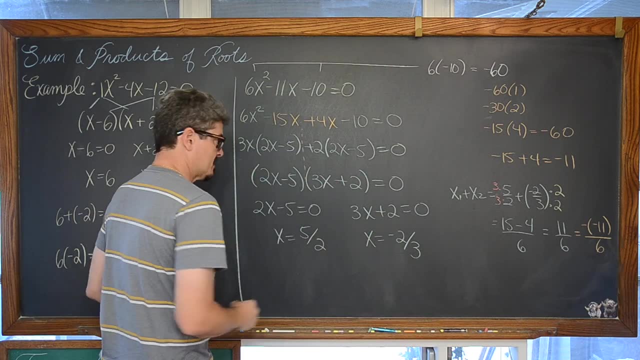 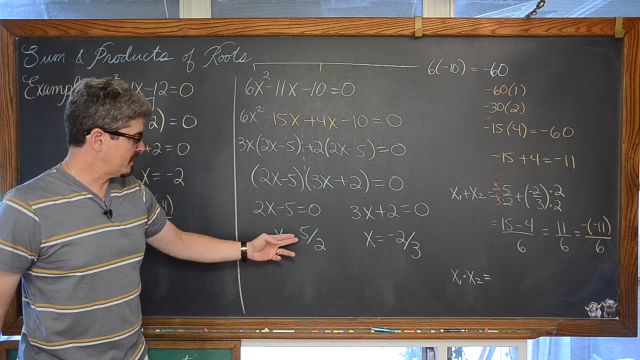 to the opposite of the coefficient of b divided by the coefficient of a. Now, if we look at the roots multiplied togetherwell, if we look at x sub 1 times x sub 2, then we are looking at 5 over, 2 times negative, 3 times negative 3.. So that is a combination of 2 over 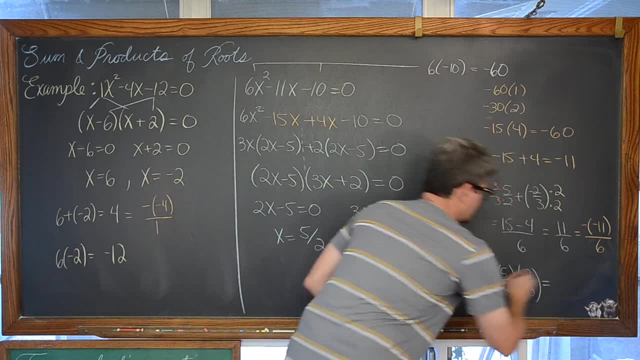 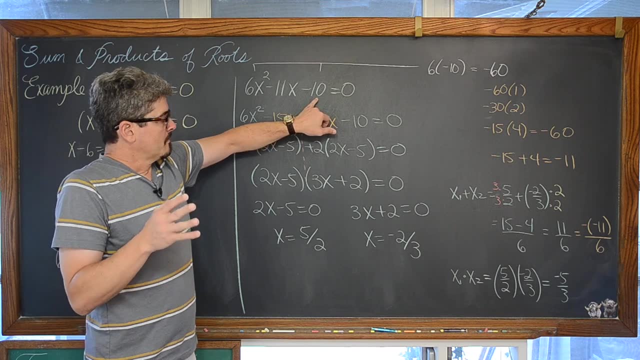 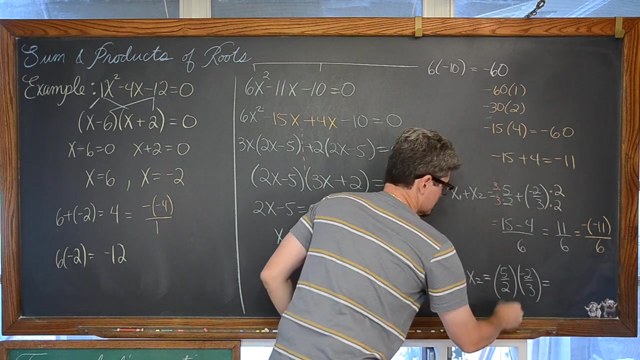 2 over 3, giving us with the 2's canceling out negative 5 thirds. Well, yeah, I'm actually kind of hiding the relationship here because I've already deduced this product as I've multiplied. So let me just really make this obvious: 5 times negative 2 is negative 10,. 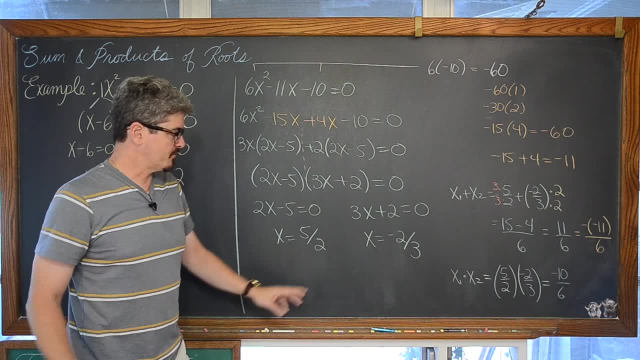 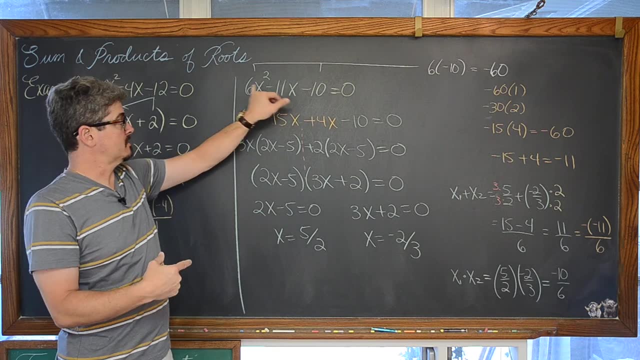 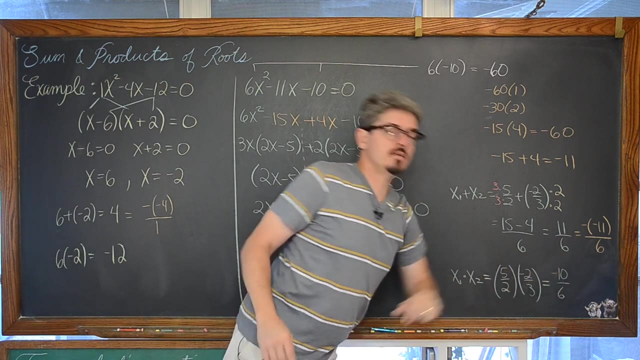 and 2 times 3 is equal to 6.. The product that you get from the two roots of your quadratic are equal to the well negative 10 divided by 6.. Actually, looking at just simply the quotient of c over a is what you get when you look at the product for the two roots. 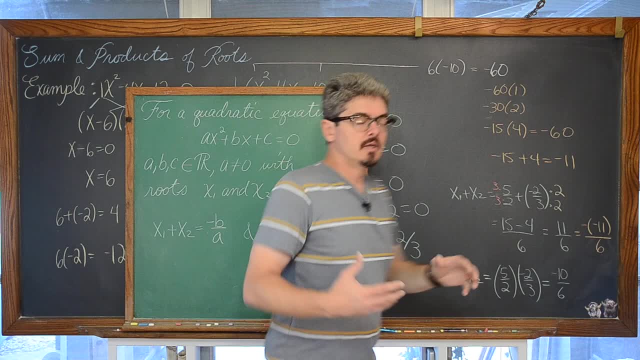 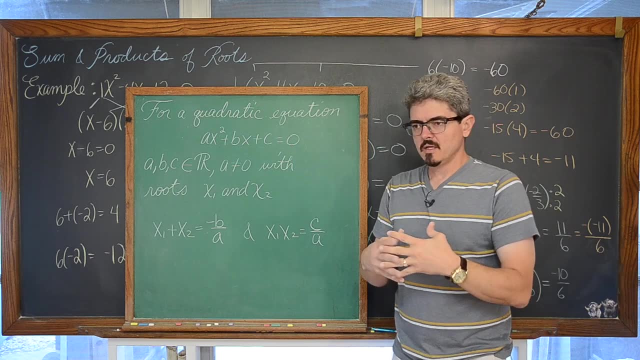 of the quadratic And that's what we're going to use to really look at the main three examples of our video. here We're going to be analyzing some products and sums and squares of the roots that we would be using to calculate the product for the two roots of the quadratic. 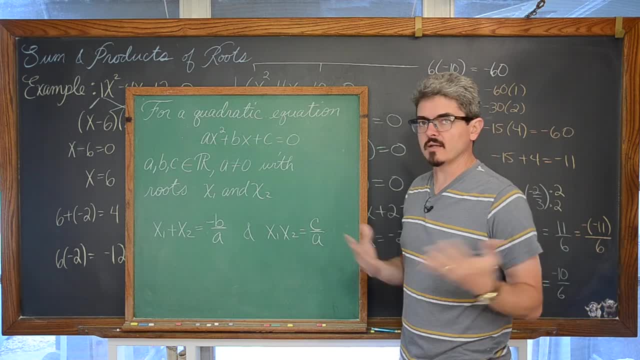 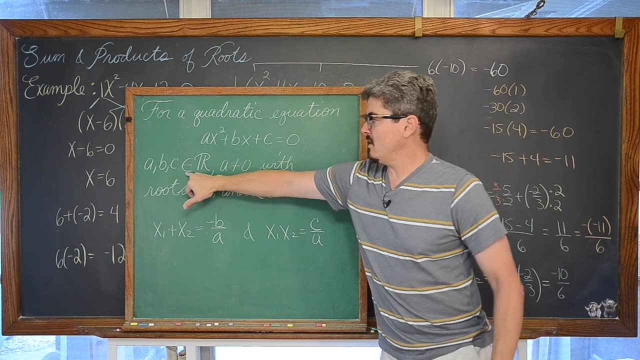 We're going to be getting from a quadratic equation without actually solving the quadratic equation. So for a quadratic equation, ax squared plus bx plus c equals zero, As long as a, b and c are elements of the real set, the real numbers, and a is not equal to zero. 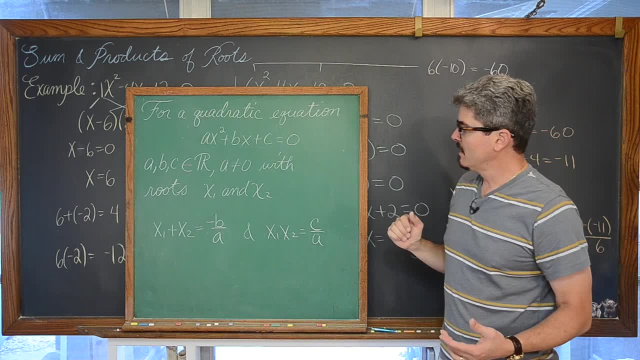 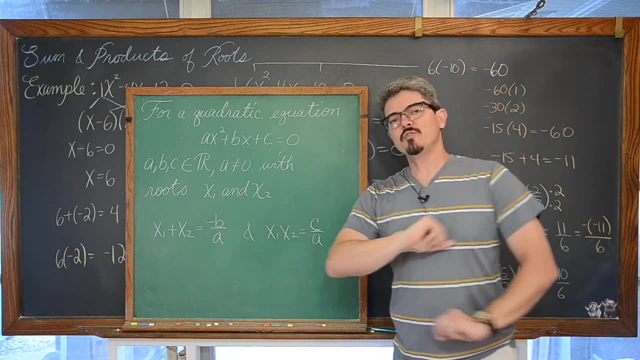 because then you would not be dealing with a quadratic but a linear function With the roots of x sub 1 and x sub 2, the sum of those roots is equal to the opposite of coefficient b divided by coefficient of a, and the product is equal to c over a. 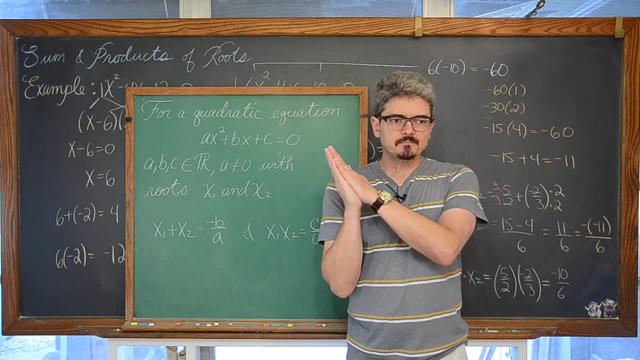 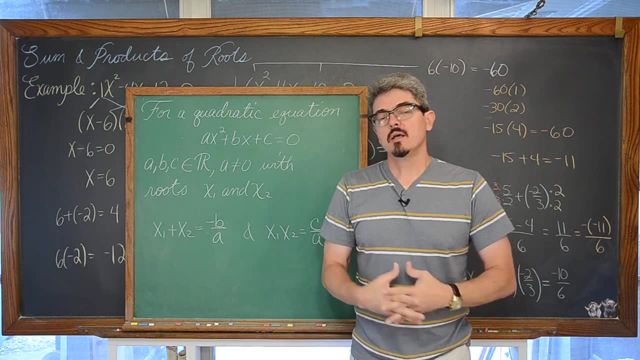 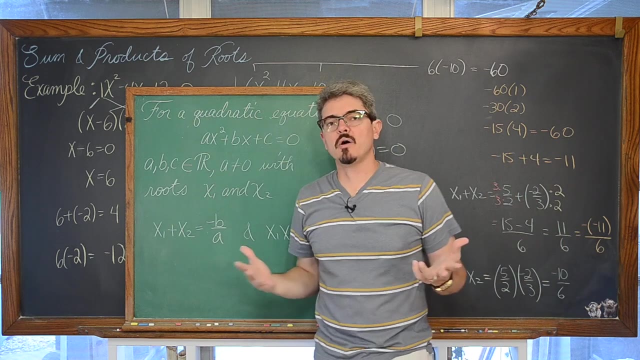 We are just going to be looking at this as just an algebraic evaluation of some requested expressions. This does extend to more than just second degree polynomials, but third, fourth and fifth and tenth, basically all polynomials. This idea can be extended to: 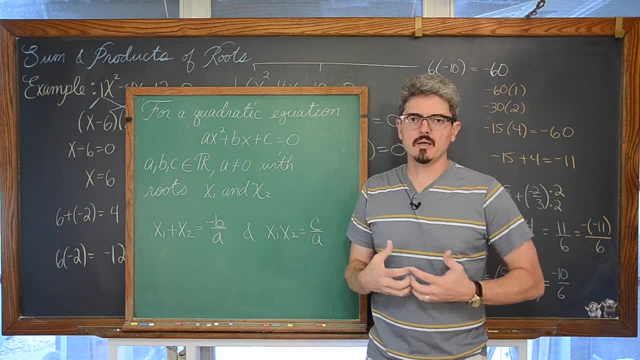 it And you'll see questions on, possibly like an IB exam that would be rooted in the foundation of knowing how or what the sum and the product of root of c are, And we're going to be looking at some of those questions after this video, But until then, thanks for watching, I hope. 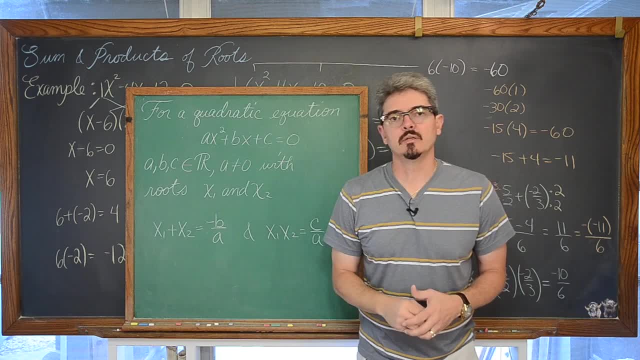 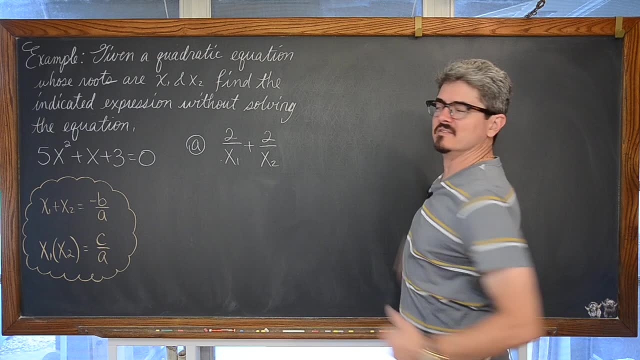 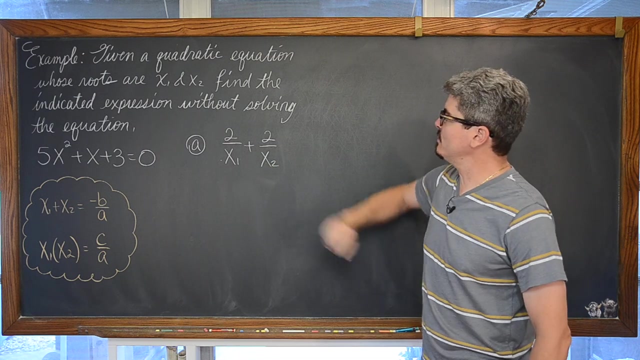 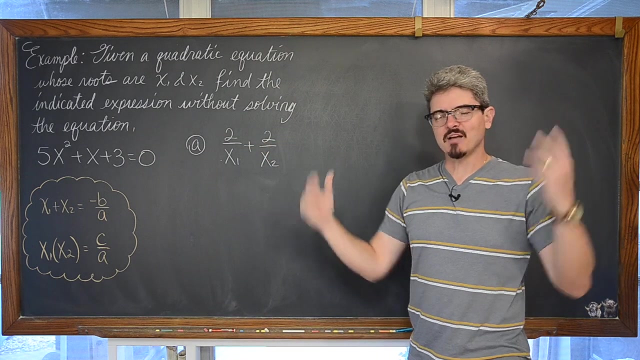 you enjoyed the video. See you next time. roots yield in terms of coefficients of a given polynomial. First example coming up right now. And for our first example, given the quadratic whose roots are equal to x sub 1 and x sub 2, find the indicated expression without actually solving the equation. Yep. 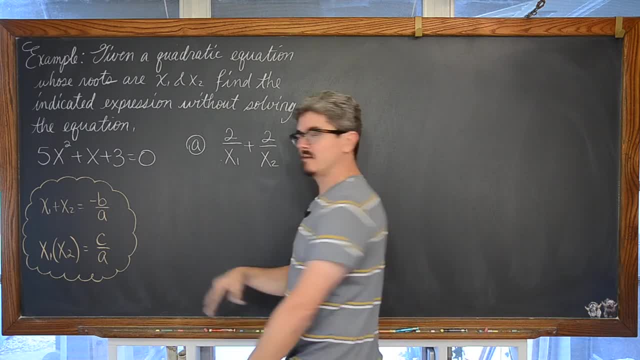 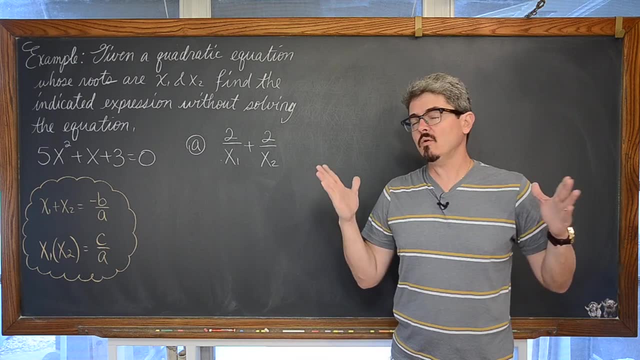 I felt that it was so important that I still went ahead and reviewed with you how to solve quadratics- especially when that leading coefficient is not equal to 1, with factoring, even though we are actually not going to solve this quadratic. to answer this question, or 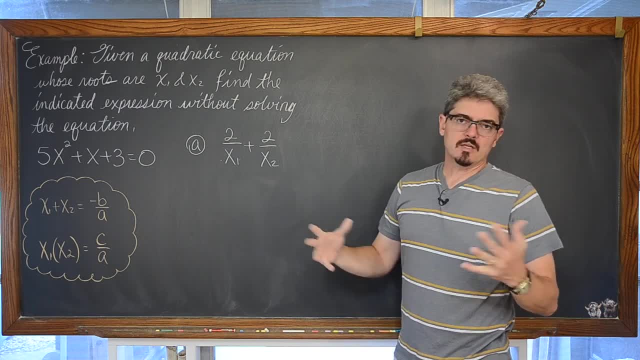 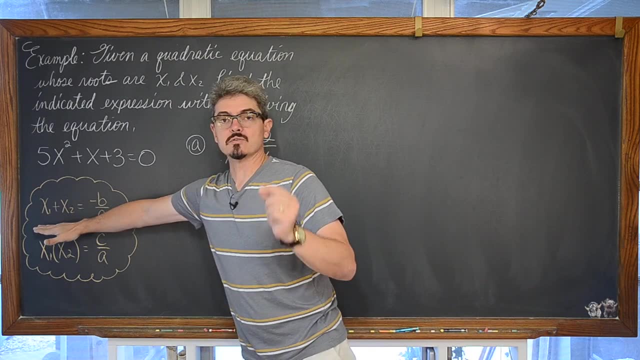 basically evaluate this expression or any of the expressions that we are given in the next three examples. I wanted you to see that review of factoring. It is really, really important and a lot of my students struggle with it And I wanted to see for yourself. 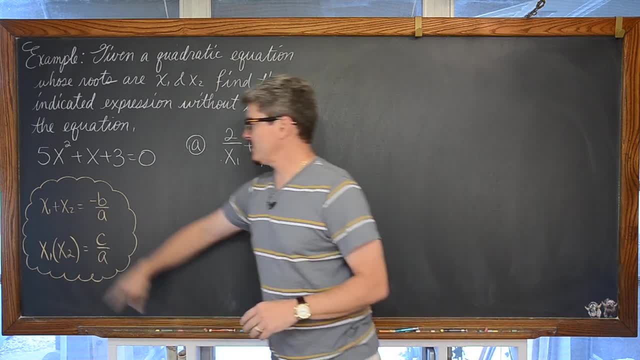 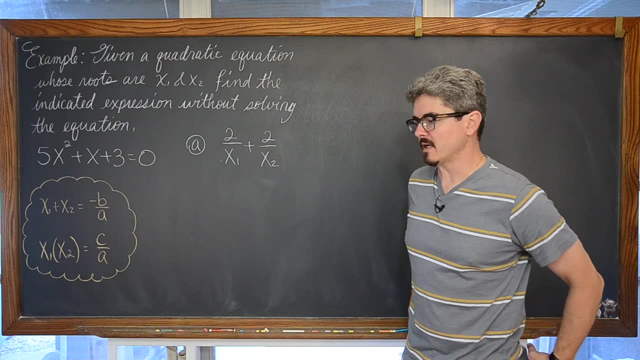 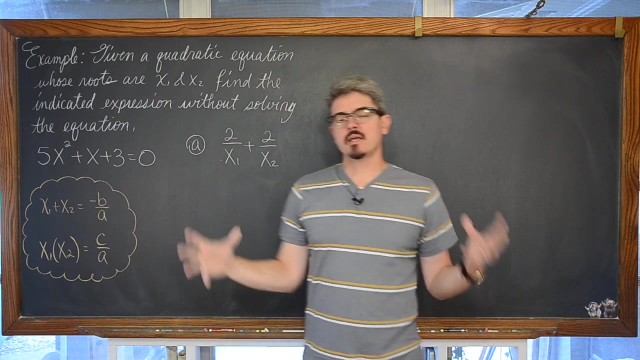 through a couple of examples- not proofs, but with a couple of examples: that relationship of the sum and the product of the sum. In the first example, with the square root and the rest of the things we are going to do, We are going to take our x sub 2, we are going to take our square root and we are going 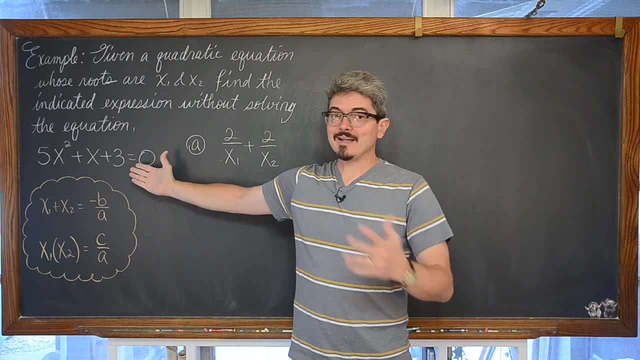 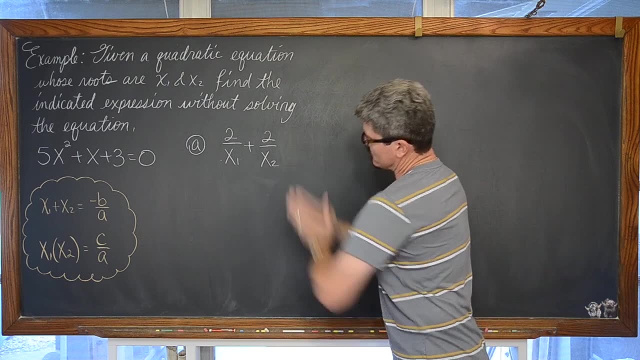 to make sure that x sub two is going to be equal to one and we are going to use the same expression, favorite, And so we want to be able to do this. Here is what I want you to do. When you two are even I don't know in terms of case by case, you can do something. 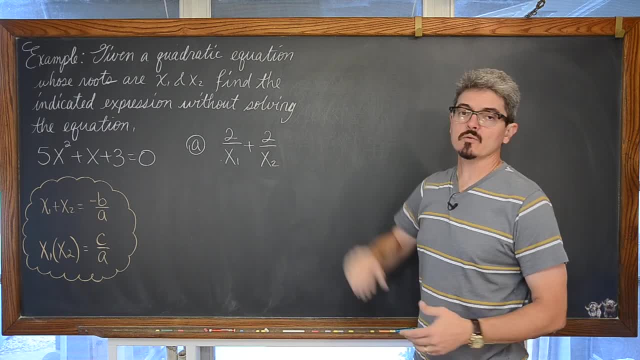 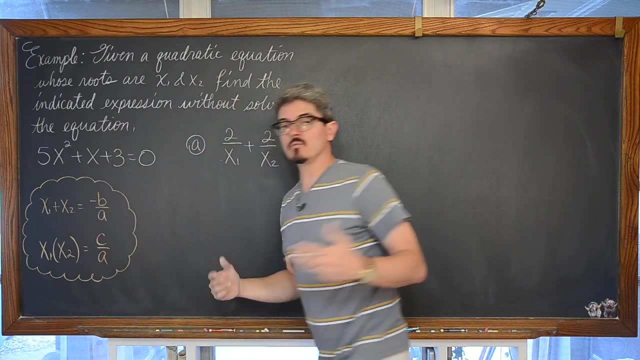 like this. I am going to do this. I am going to take my square root and the plus sign that, knowing the roots that you know that we could just easily substitute in here and get the same answer. what if it was a fourth degree and I didn't want to? 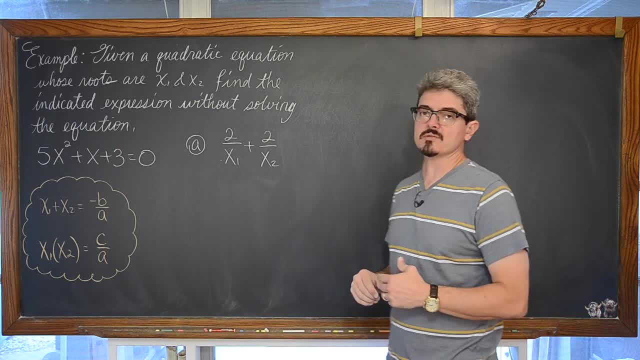 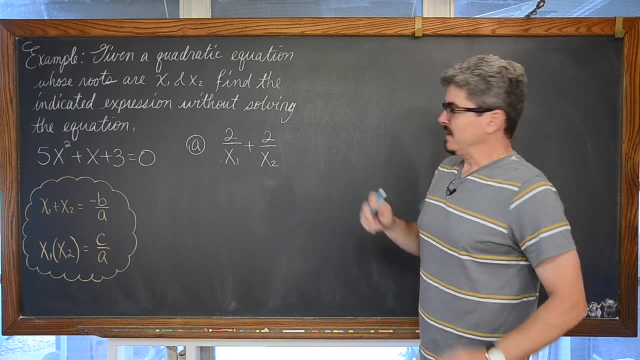 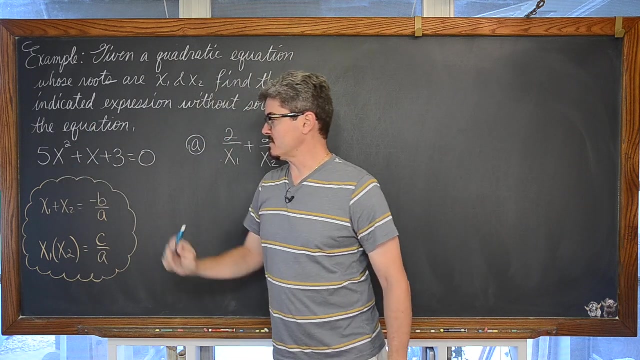 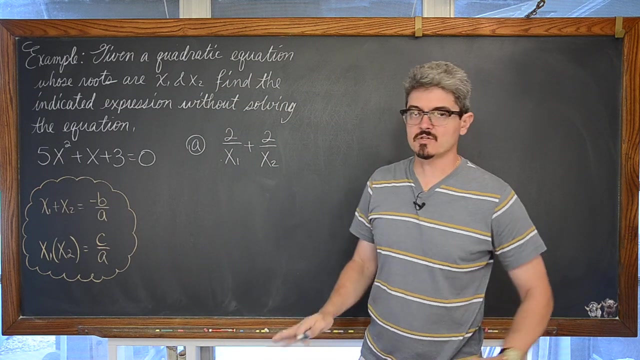 actually solve that higher, higher order polynomial. I could still evaluate this expression. so don't resist solving that quadratic, even though we can easily. the relationship of our roots to this polynomial and the coefficients is based only on sum and product, not subtraction, not division. so if I can't rework this, 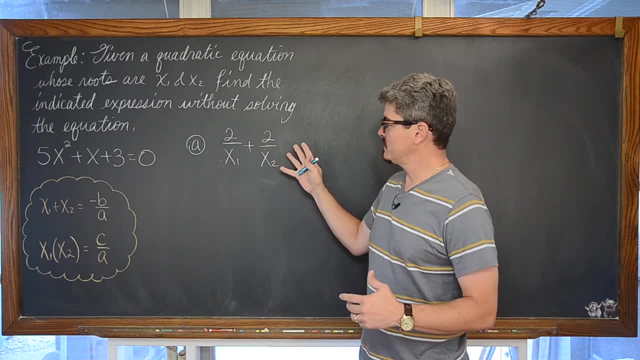 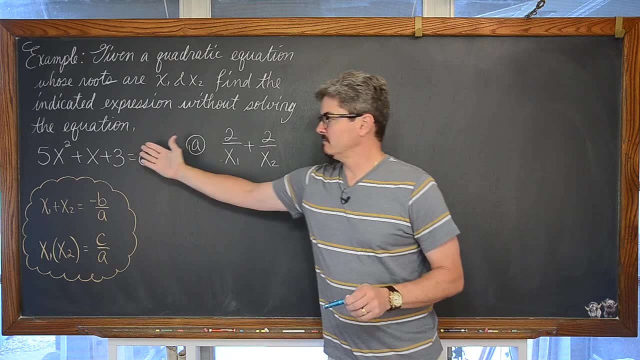 expression a little bit to develop a sum and product of these roots of X sub 1 and X sub 2. we're not going to be able to evaluate it, at least not without relying on solving this. so how are we going to manipulate this expression to create? 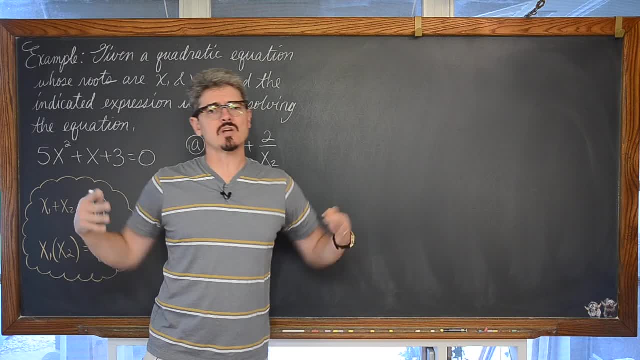 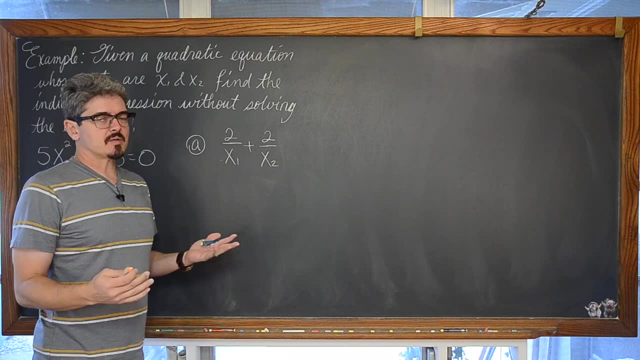 some sums and products of roots. well, just try something like you did in your geometry two-column proofs or your trig proofs and pre-calculations and so on and so forth. so what we're going to do is we're going to do some algebra and see if something nice happens, like we have two terms. 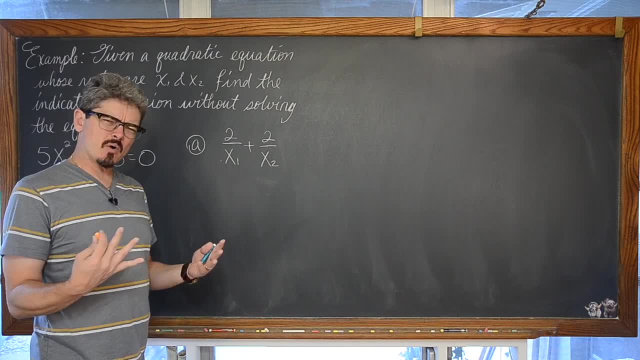 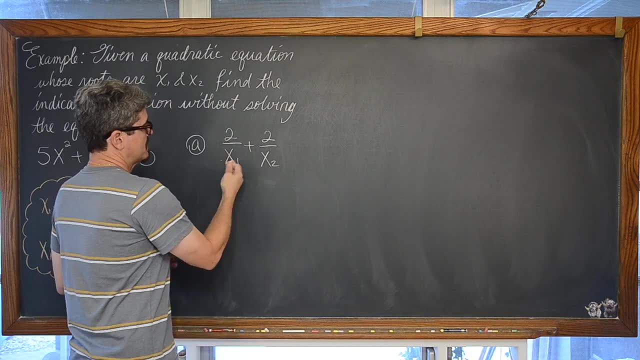 maybe we could add these two terms and make one fraction that requires multiplication through the process of finding common denominators. maybe that'll help. so we have a factor, or basically a factor of X sub 1, a factor of X sub 2- we're assuming these having no common factors, because, of course, how would we 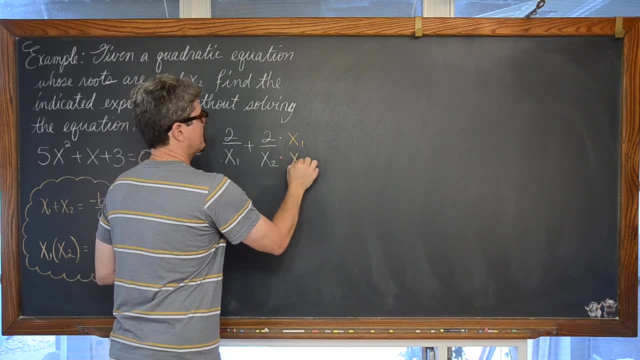 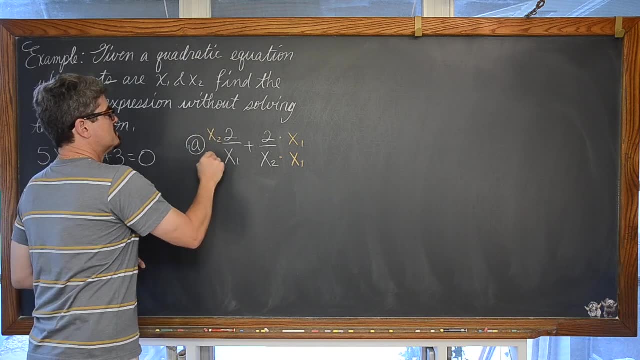 know we're gonna multiply the numerator and denominator by X sub 1 here, because anything divided by itself is 1, so we're just going to change the way it looks. what do we get? we have two times X sub 2 plus 2 times X sub 1. that's our. 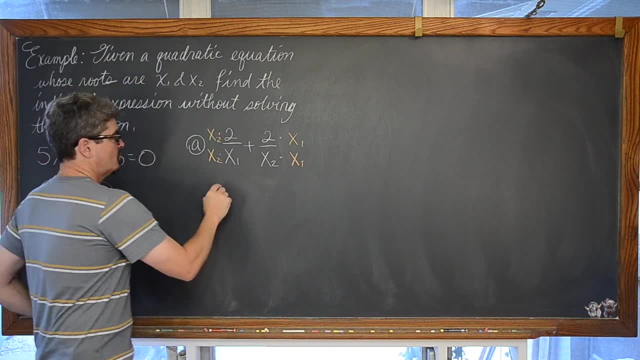 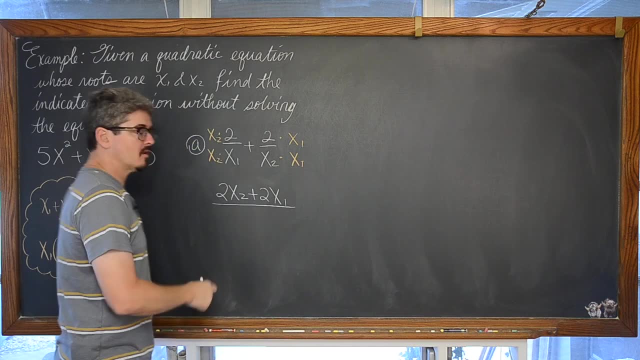 numerator, I'm gonna write a big old fraction bar because while we just created that common denominator that we need it, there's the product in the denominator that we need. so ultimately, this is going to get pulled out and be sub and be replaced or substituted in plus X and 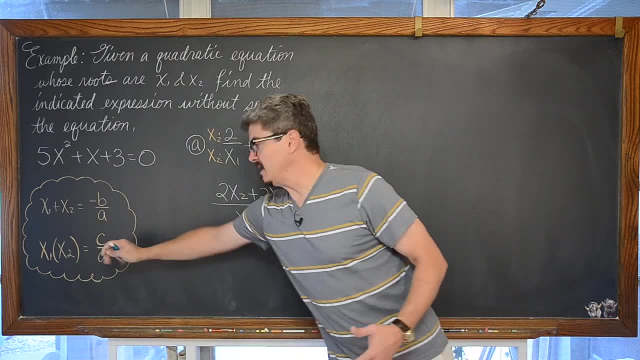 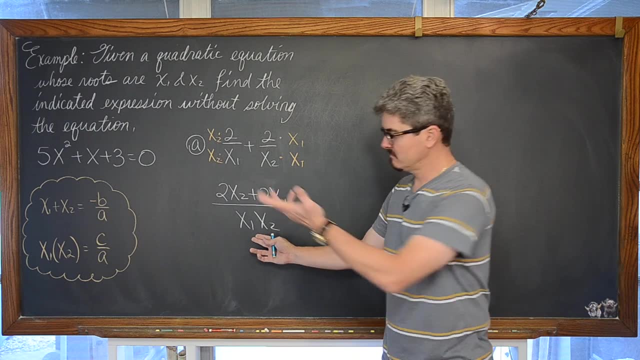 we now, we, that's our slot. so the essentially where it takes the numerator and sub, that's the denominator we need to replace in, and so we're going to list, substituted in place of this product, The coefficients of c divided by a. We are almost. 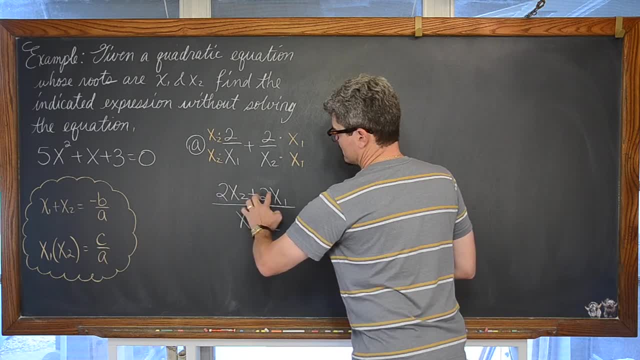 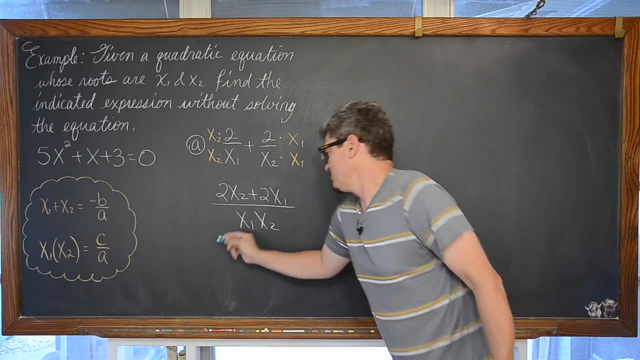 done. of course We are ready for that substitution, But we do want to get this pesky coefficient of 2 out, So we just have that x sub 1 plus x sub 2.. So yeah, just factor it So 2 times. 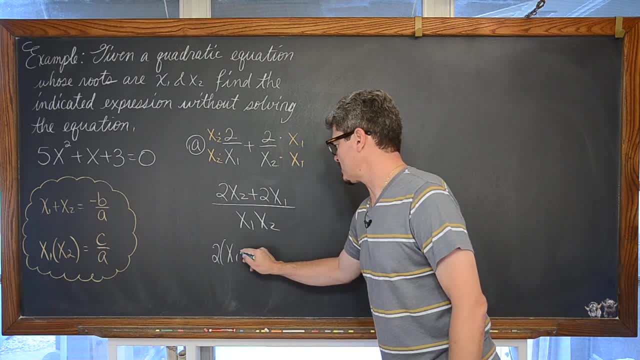 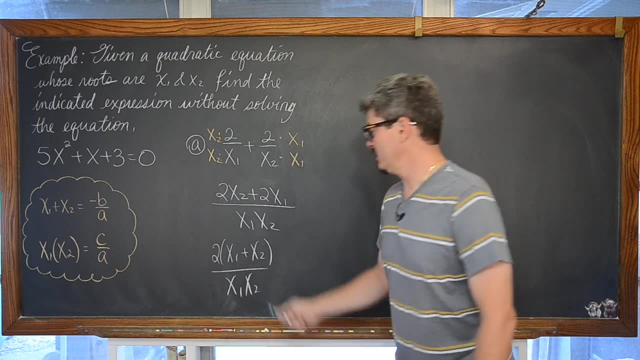 x sub. This is addition, so it is commutative. I am just going to turn this around: x sub 1 plus x sub 2, over x sub 1 times x sub 2.. There is our sum and product of our roots. 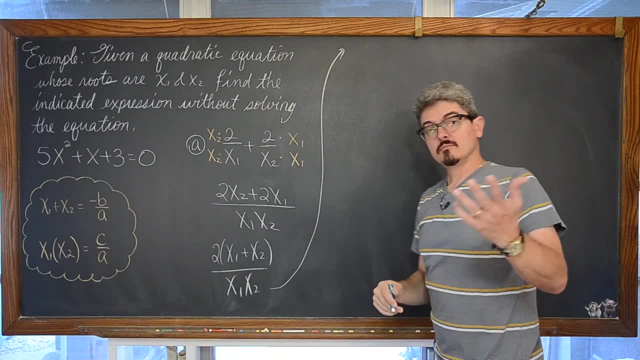 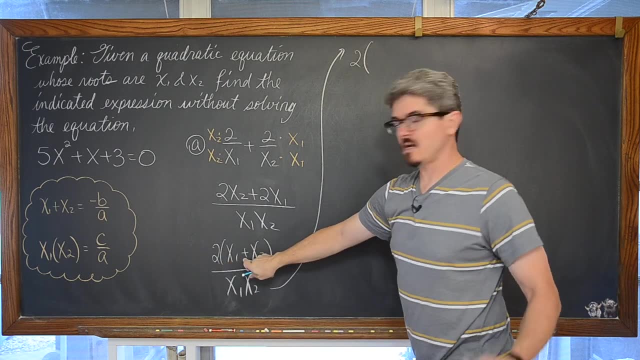 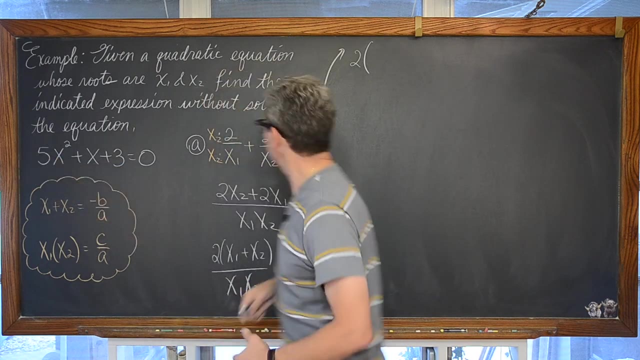 for this quadratic. So we are ready to substitute and just simplify What is left. We have 2 times the sum of our roots, which is the opposite of coefficient b over coefficient of a. So it is the opposite of 1 over 5.. 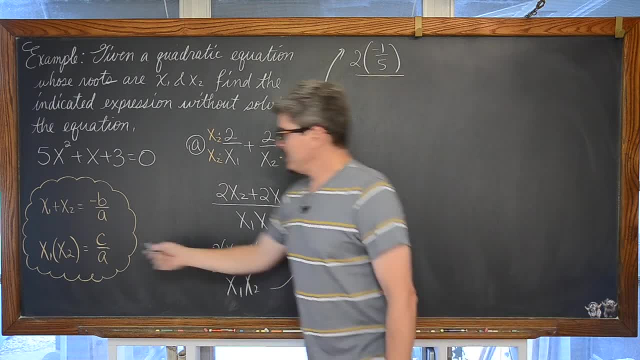 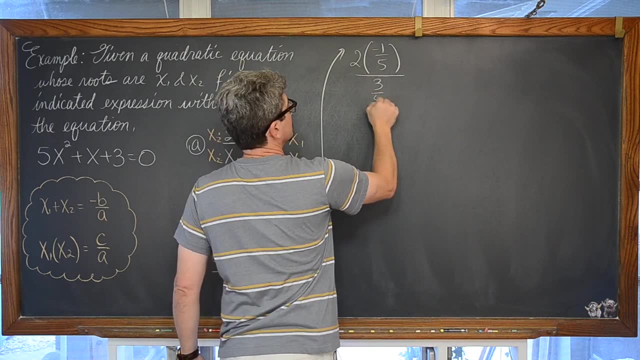 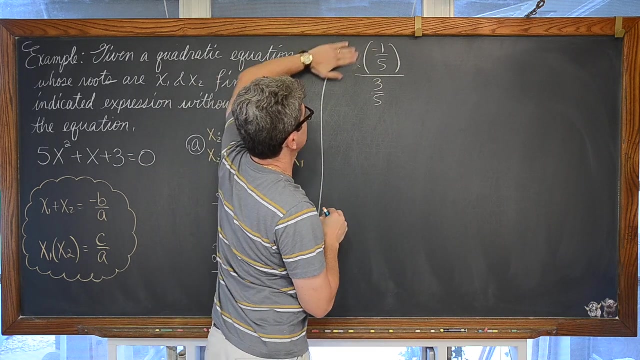 Divided by the product, which is going to be equal to the quotient of the constant divided by the leading coefficient. So over 3 fifths, And hopefully you are good with fractions by now. I don't really know what math class you are studying at the moment, but this is 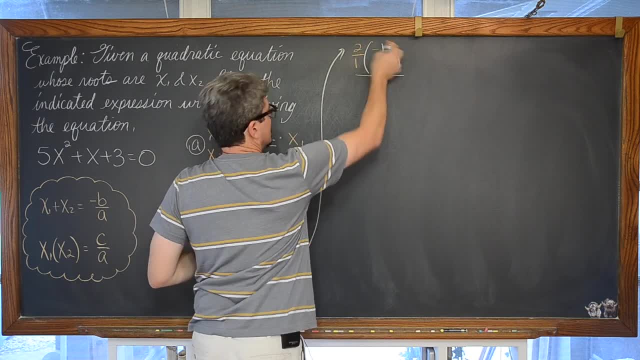 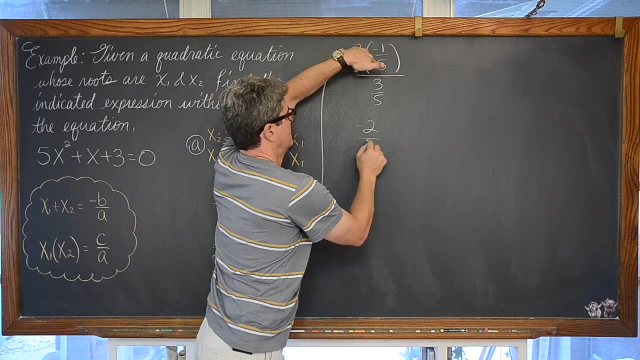 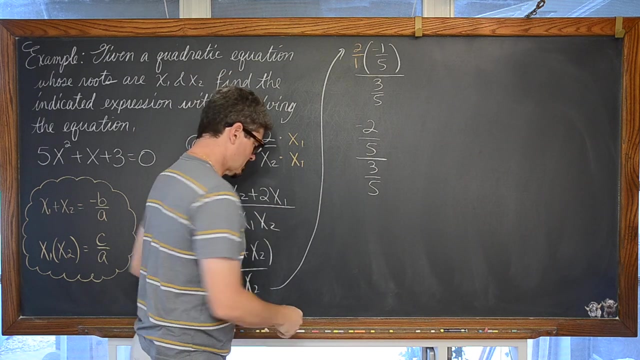 2 times negative 1 fifth, or 2 over 1 times negative 1 fifth. So we are going to multiply the numerators, We are going to multiply the denominators, So we have negative 2 fifths Over 3 fifths. You may know that these common denominators, the denominators of 5 in the 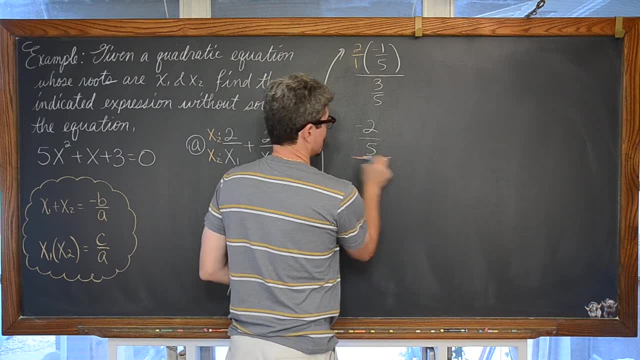 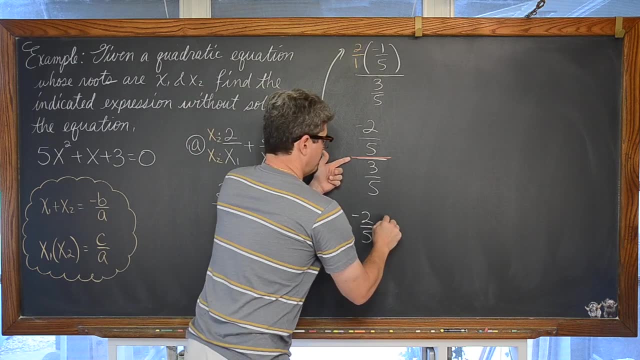 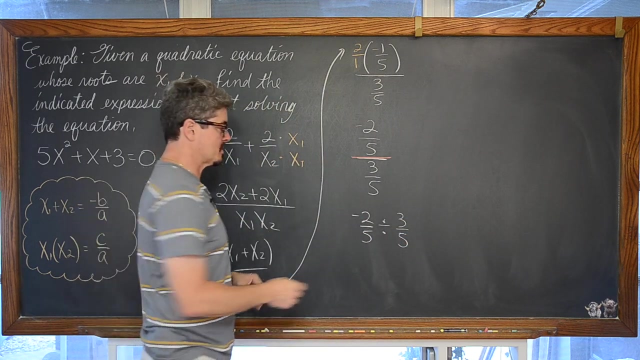 numerator and denominator are going to cancel, But just in case we have our main fraction bar. here We have negative 2 fifths divided by our denominator of 3 fifths. Of course we don't really divide fractions, We multiply by those reciprocals or the reciprocal of 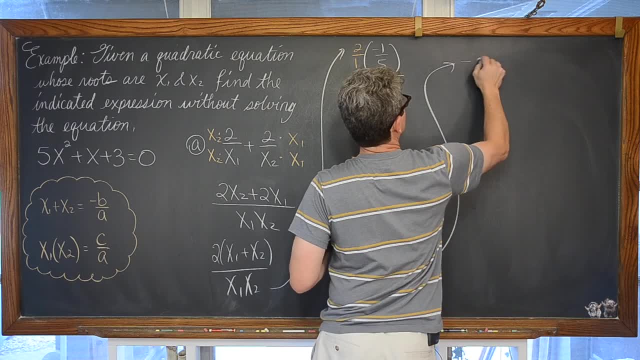 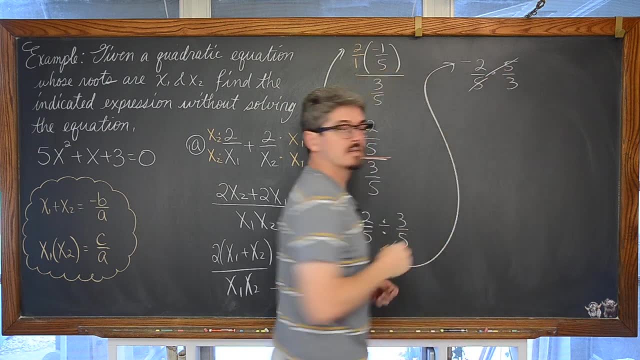 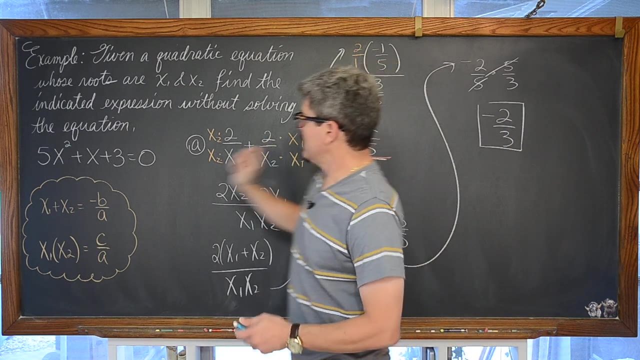 the second factor. So we are looking at negative 2 fifths Times 5 thirds. 5 divided by 5 is going to cancel And we have negative 2 thirds. So, given that- and double check, yes- So given that we have this quadratic equation, 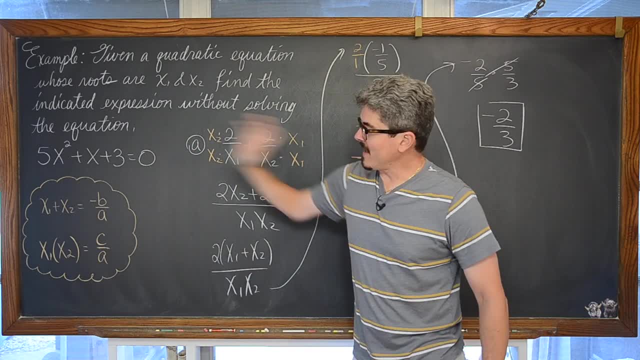 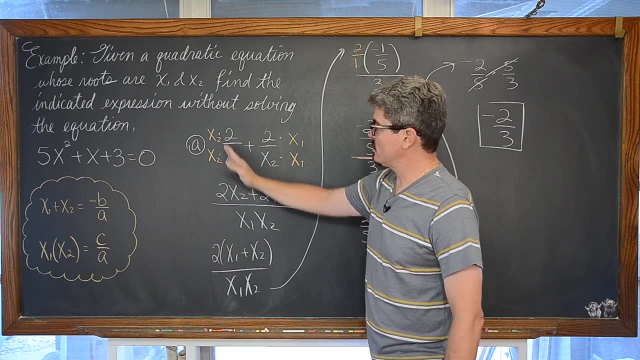 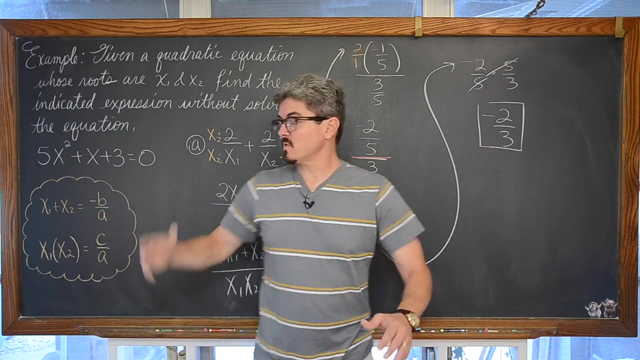 of negative 5x squared plus x plus 3.. And without solving that, because maybe with a higher order polynomial it would be very hard to solve, We are going to evaluate this expression, The expression of 2 over x sub 1, plus 2 over x sub 2. Turns out that it is equal to 2 thirds. 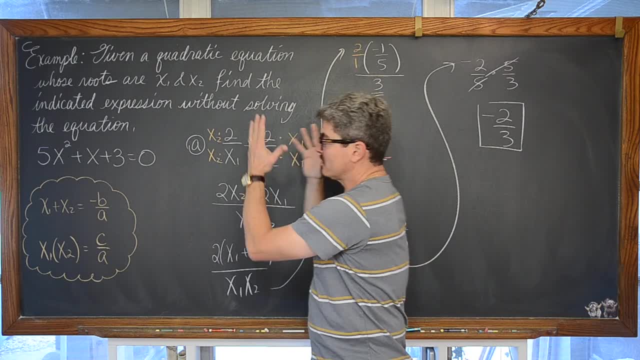 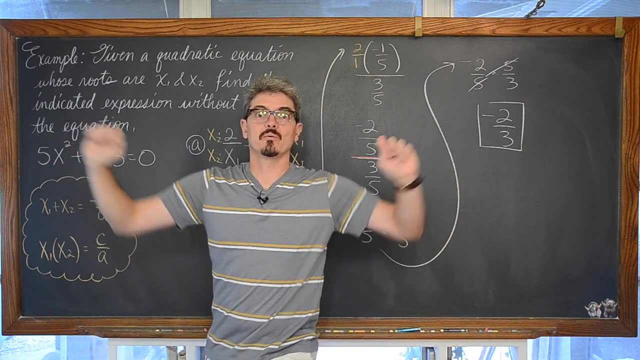 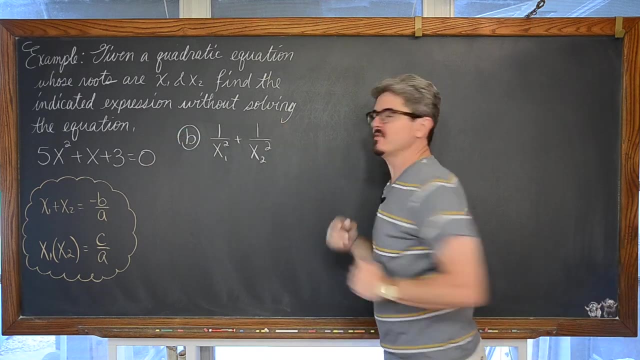 So I could evaluate some expression based on roots of this polynomial without having to solve that polynomial. Very, very cool. I have two more examples coming up right now. No, no, no, no, no, no. Alrighty, then We have the same quadratic and we have a different. 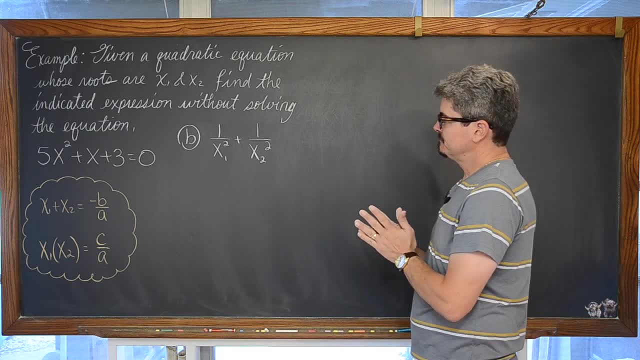 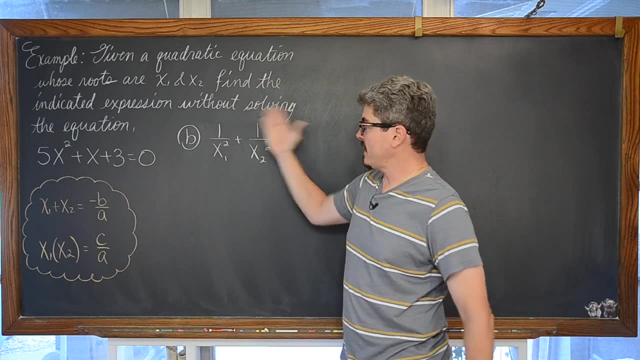 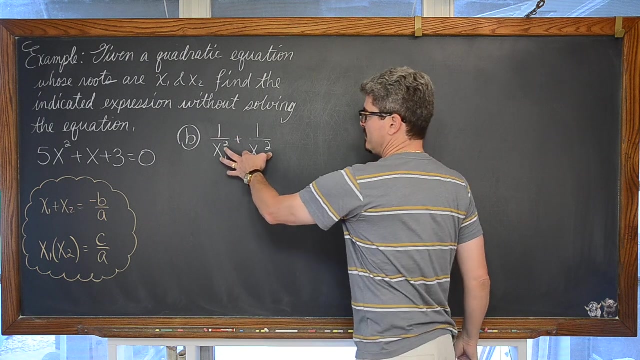 expression that we are going to evaluate Again, some End product All we can look at or that we need to develop out of this expression, And there are no powers of 2's on any of those terms. So we have possibly a bit of an issue. 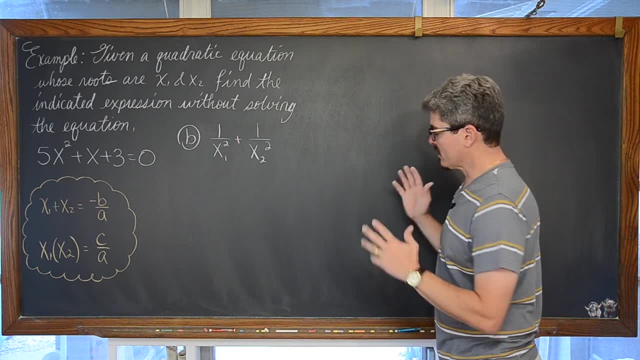 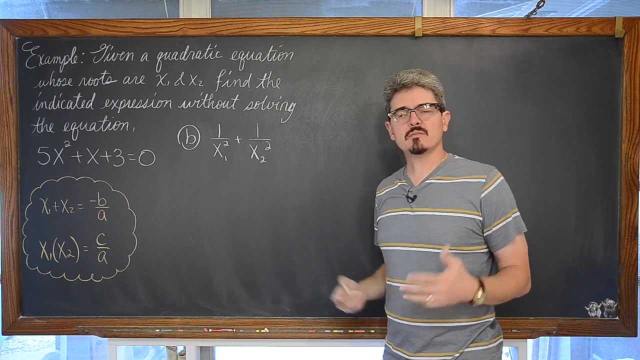 the fact that x sub 1 is squared and x sub 2 is squared. We are going to go through the same process of finding that common denominator, though, because we have our two separate terms, And adding two fractions and making one sure worked on the first example. So let's give 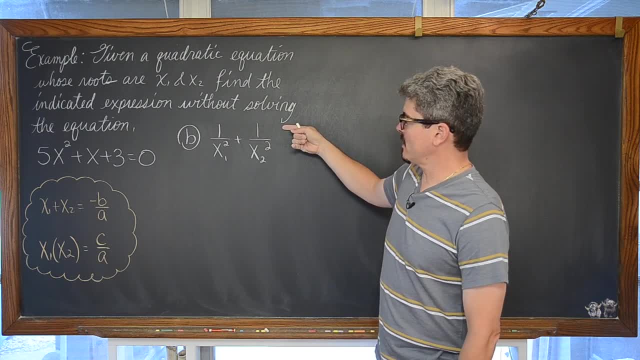 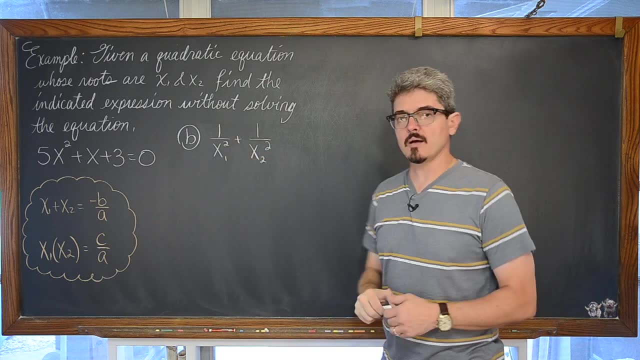 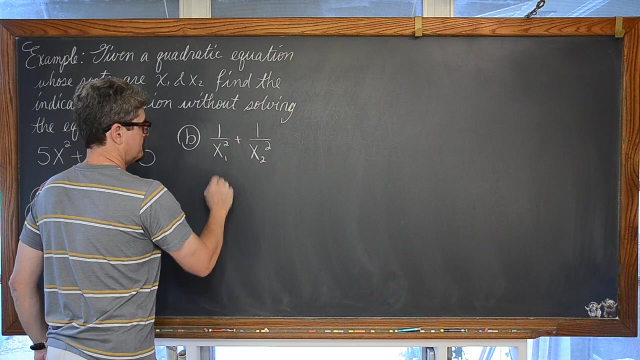 it another try. We are going to multiply x squared or x sub 1 squared to the numerator and denominator And x sub 2 squared to the numerator and denominator as well, And that is going to give us x sub 2 squared plus. and remember, we are going 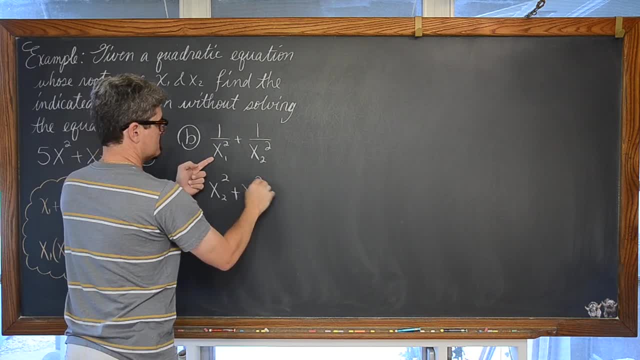 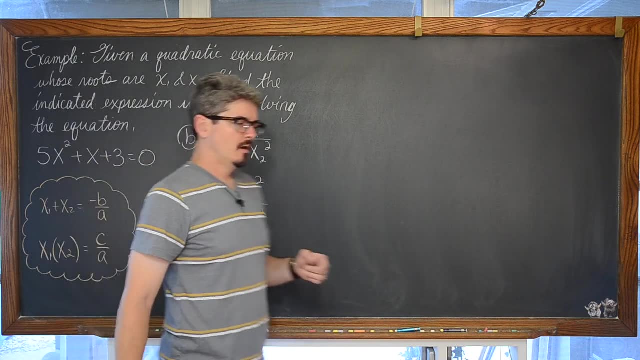 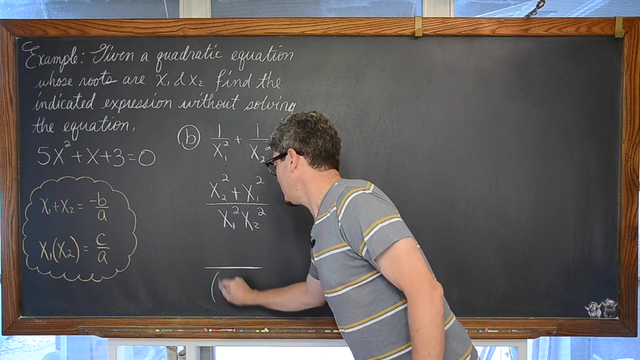 to bring this over numerator and denominator. So plus x sub 1 squared over x sub 1 squared, x sub 2 squared. Well, dealing with that power of 2 in the denominator is, I don't know, really actually quite simple. Let's just write it as x sub 1 times x sub 2 squared. 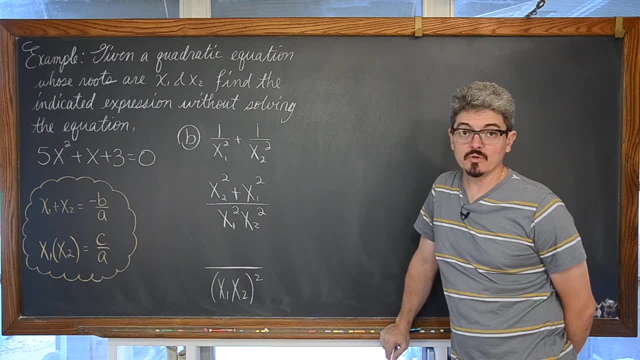 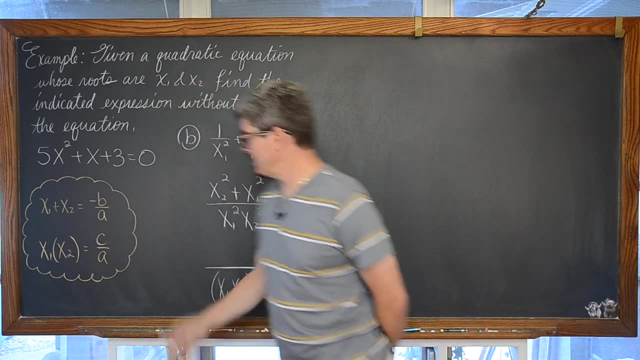 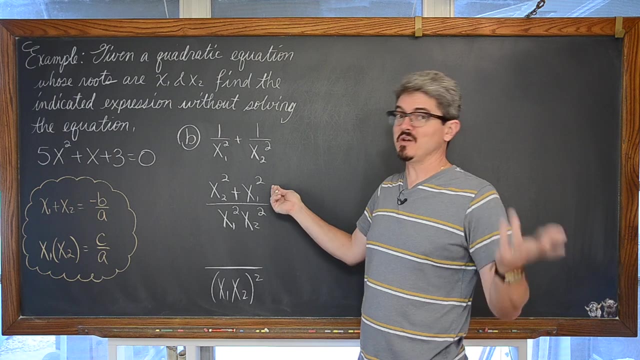 We are going to have a bigger issue in the numerator though, because powers of 2 on our sum powers of 1, this is not equal to negative b over a. it is not equal to good lord knows what my kids have come up with. it is not negative b over a squared- Yeah, It is. 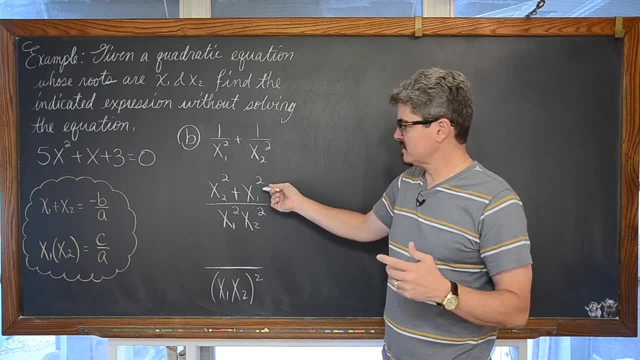 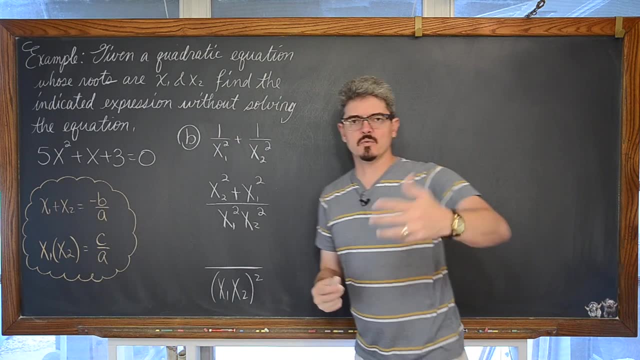 It is also not factorable. You think, well, ok, because that is how you bring exponents down, is with factoring or division, and we need to get these factors of two down to factors of one. That is something you have to deal with in your trig proofs in pre-calc. 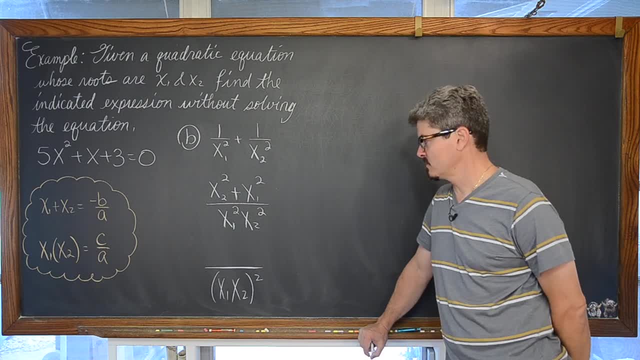 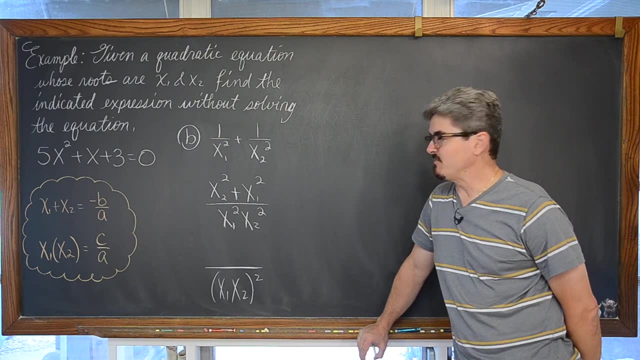 Well, if you took trig in your pre-calc class, a lot of students do just take trig as a semester course. But at any rate, I digress. I need to make something, a factorable, something quadratic that is going to go down and give. 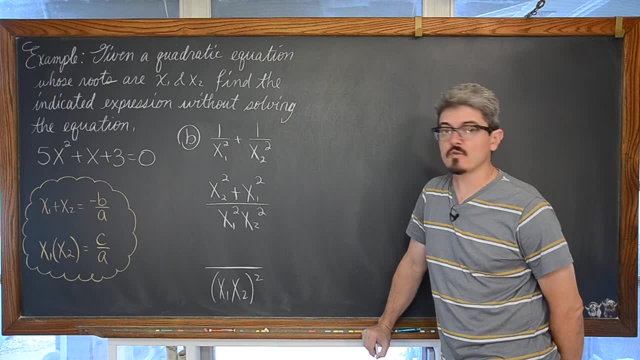 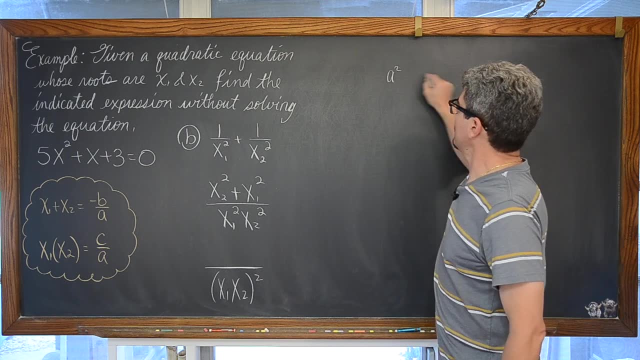 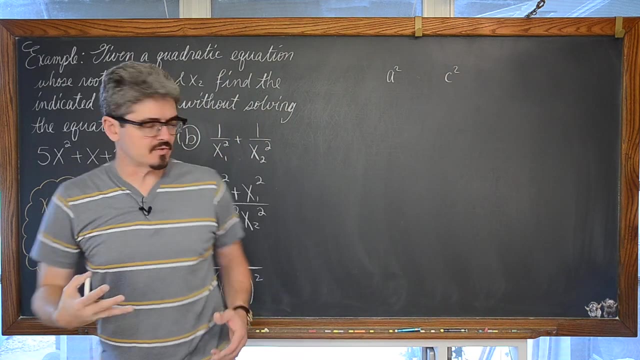 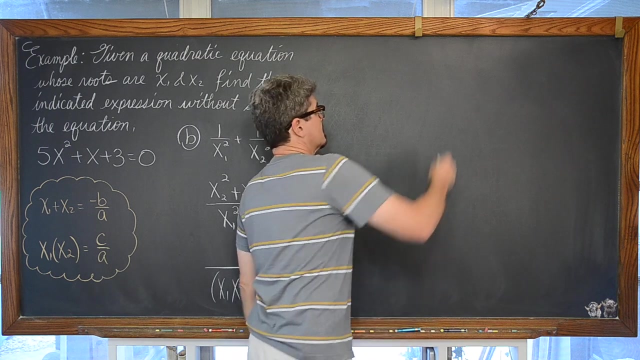 me some factors basically that are first degree. Let's see If I have a squared and c squared, what would need to be in the middle that would allow me to factor or have some kind of factorable trinomial. You know, it really kills me that all the time I get kids writing things like this: 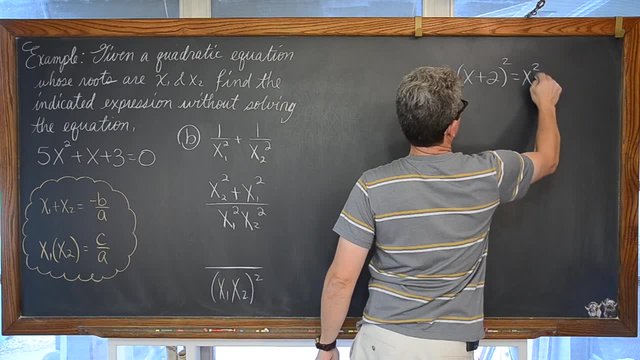 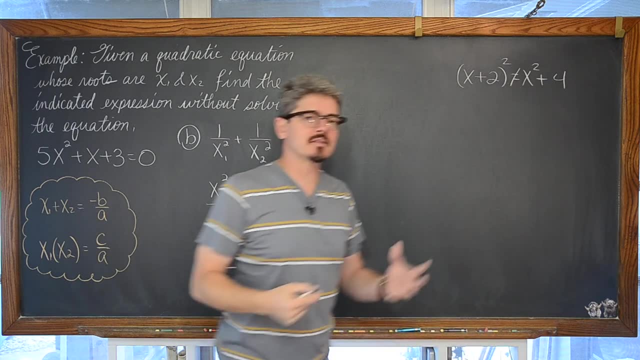 x plus two squared. is x squared plus two? Well, four, because I do two squared and I go no, no, no, come on, you are making me just die a little bit inside. When you square a binomial, you are supposed to have three terms. 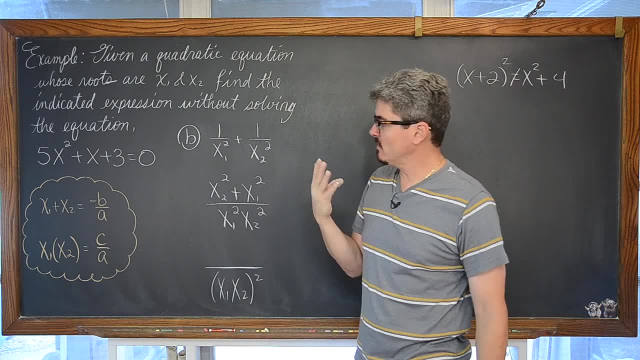 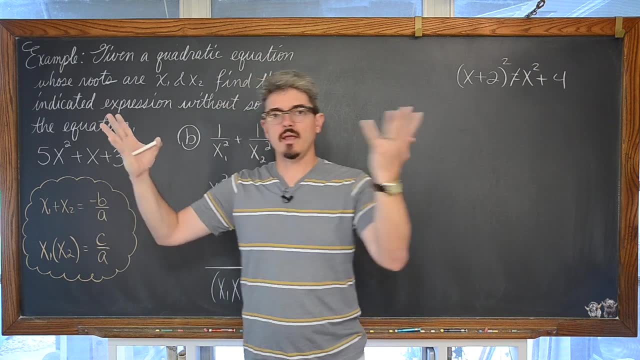 Unless it is, yeah, any binomial squared is three terms And you know what? I need to have an x, basically x sub one plus x sub two somewhere. So like, basically, let's go ahead and write this: How about we just write this? 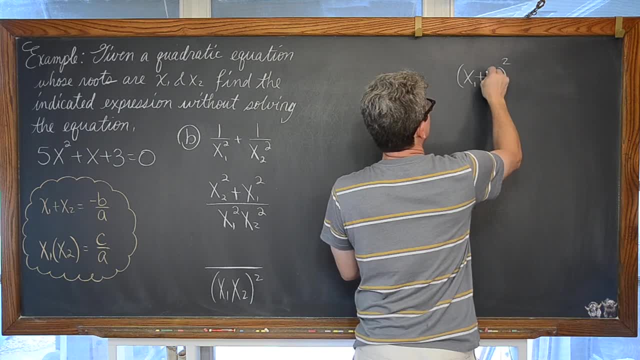 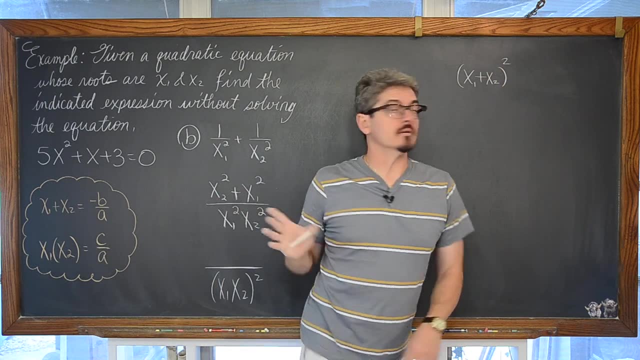 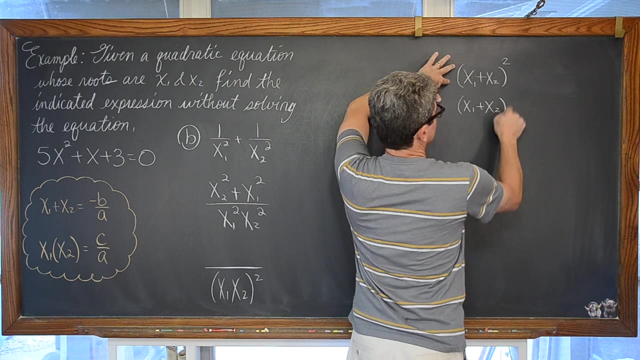 x sub one plus x sub two, with a power of two on it. Why? Because I have powers of two in my numerator. If I expand this binomial out, we are going to get x sub one plus x sub two, x sub one. 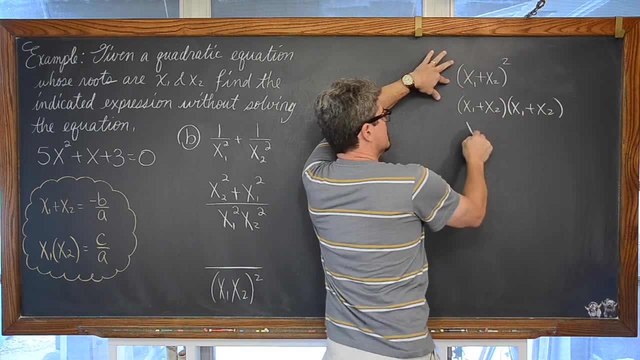 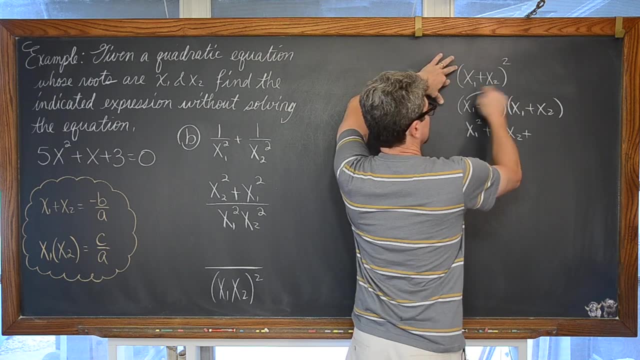 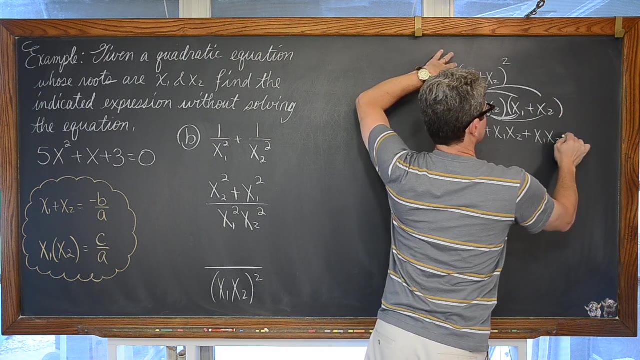 plus x sub two. x sub one times x sub one is x sub one squared. x sub one times x sub two is x sub one. x sub two. x sub one, x sub two, and then x sub two times x sub two is x sub two squared. 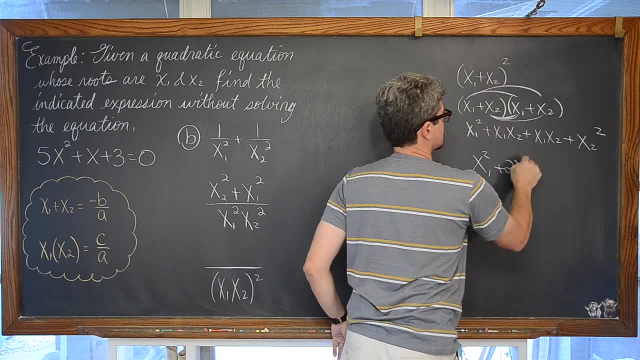 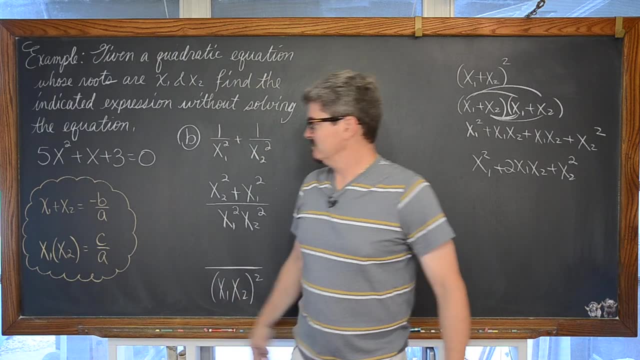 So x sub two, x sub one squared, plus two x sub one x sub two plus x sub two squared. Maybe your book would be nice to you and do something like I don't know, a plus b or u plus v or something like that. 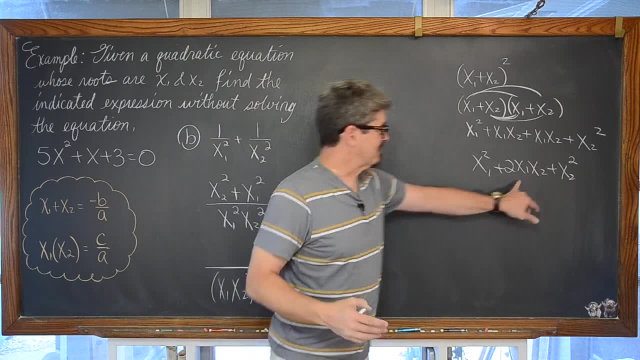 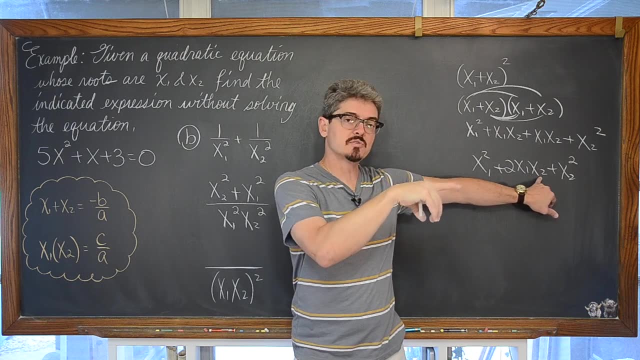 But my book- and I am staying consistent with it- uses subscripts, So this is getting kind of ugly. But look here: If I add in a plus two x sub one x sub two term, then I can take these terms that are: 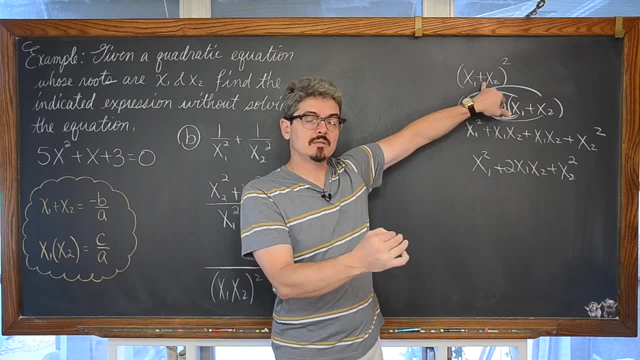 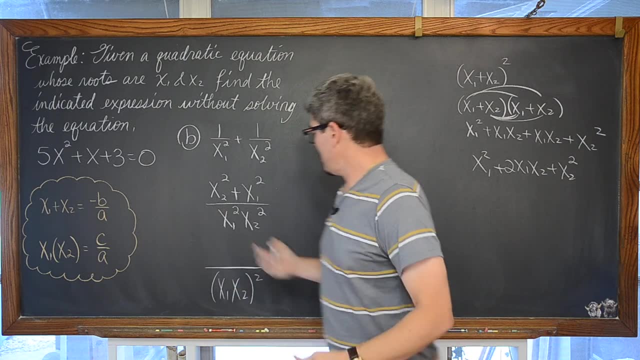 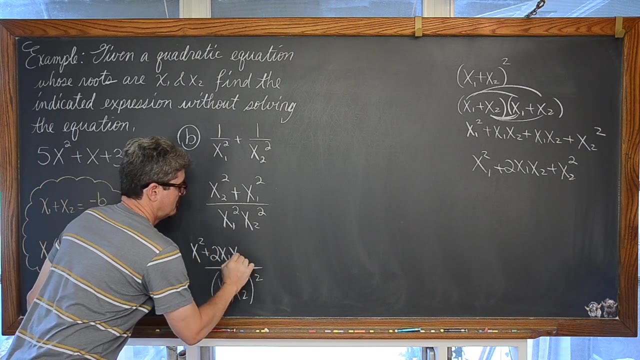 squared and factor it and get a sum of roots squared. And that is awesome, because then I would know that that sum of roots is negative b over a. Well, ok, I just need to add in another term: Ok, Ok, Ok. 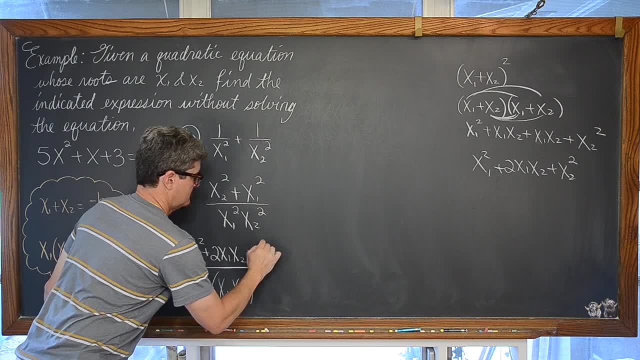 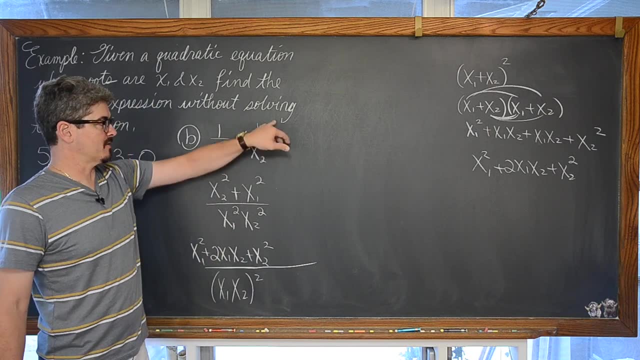 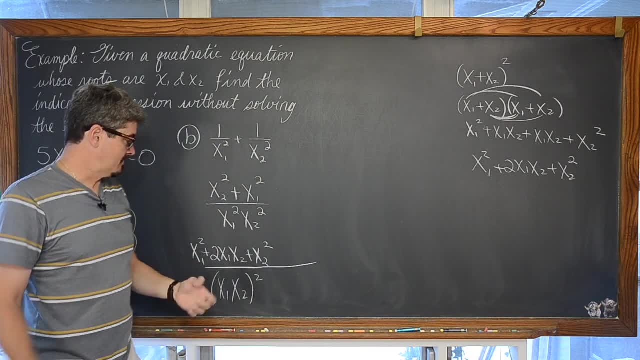 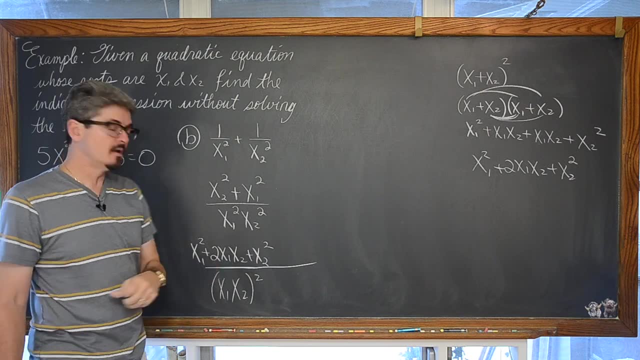 I had to multiply the numerator by a factor as well, so I would create that identity. I don't want to add in two something, I want to basically add zero. So if I am adding 2 x sub one x sub two, I need to subtract. 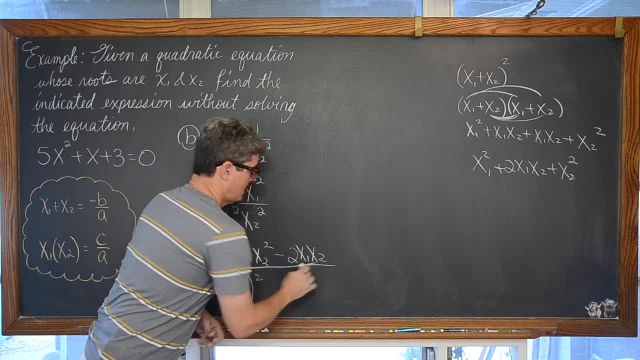 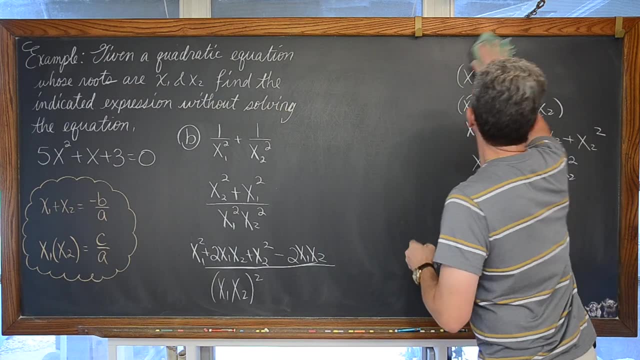 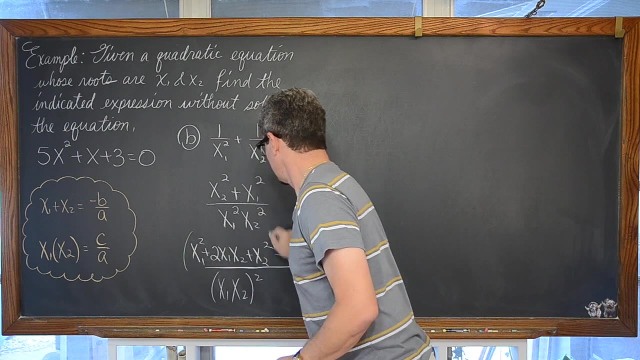 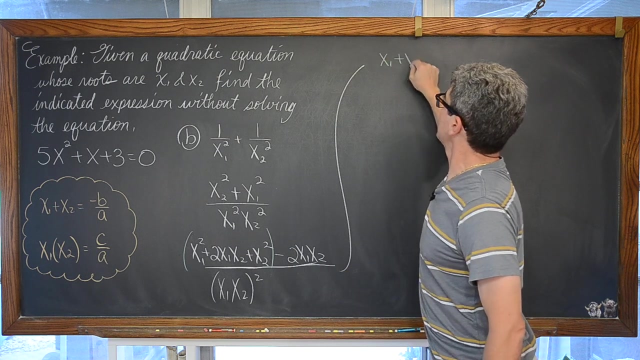 2 x sub one. So I changed the way the numerator looks, but not its actual value. Now, through my little bit of work over here, or just your vast algebra knowledge, we see that this is factorable and it is well. let's just do it in green: x sub one plus x sub. 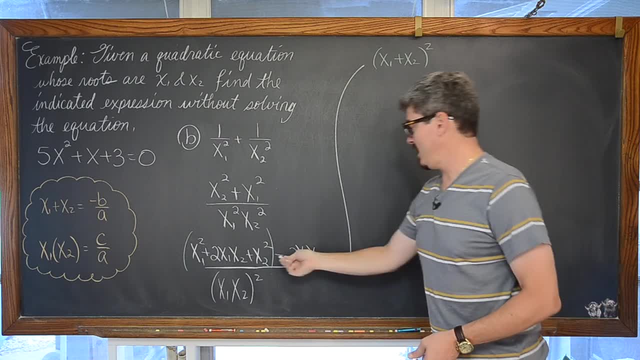 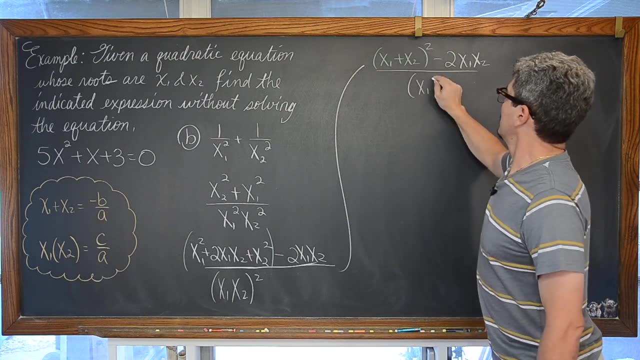 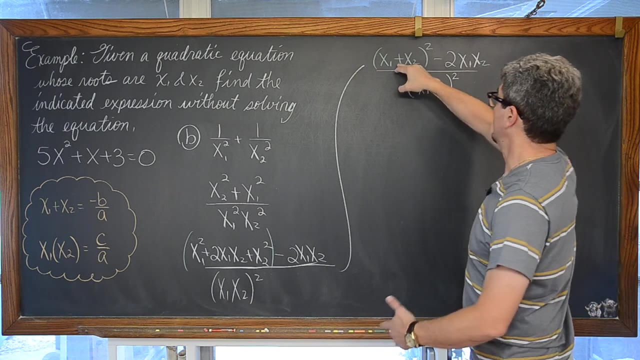 two squared. Now I have a minus two x sub one, x sub two. keep wanting to write x and y, x sub one times x sub two squared in the denominator. and now I'm at a point where, hey, I have a sum. 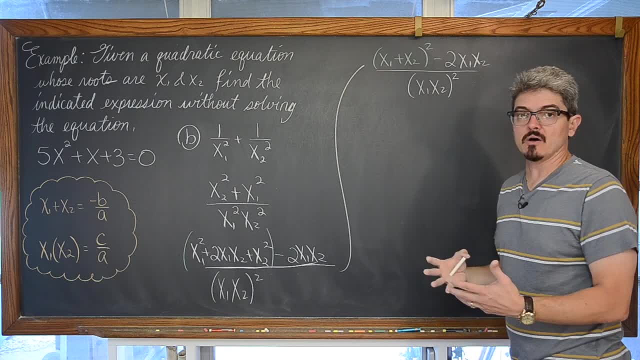 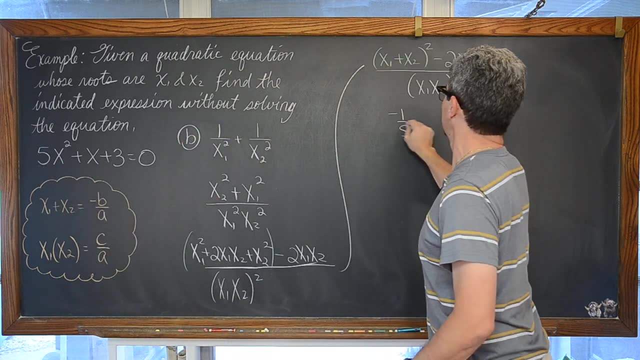 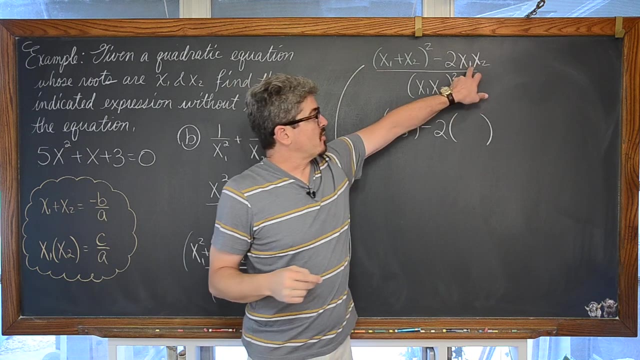 and I have a product of my roots and there's no other mess going on. then the sum of these roots is negative b over a. so we're looking at negative one fifth squared, and now we have minus two. We have a product of our roots which is equal to c over a, which is equal to three over. 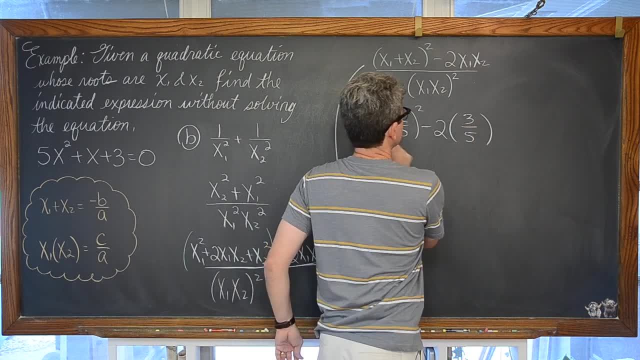 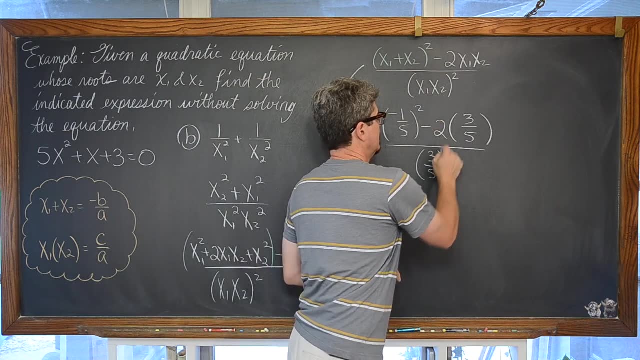 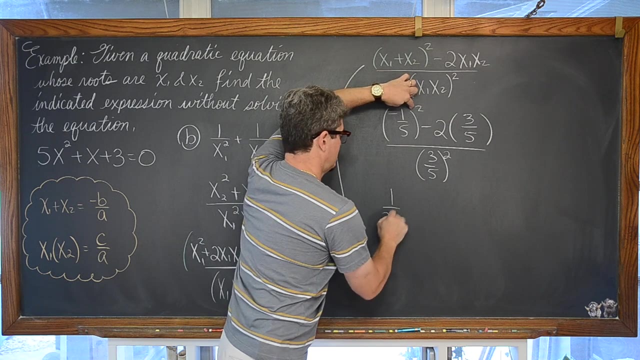 five. and yes, I picked examples that we could practice our skill of fractions. Again, we have our product. so c over a, three over five, and it's squared, So negative. one squared is one, five squared is twenty five. we have minus and this is: 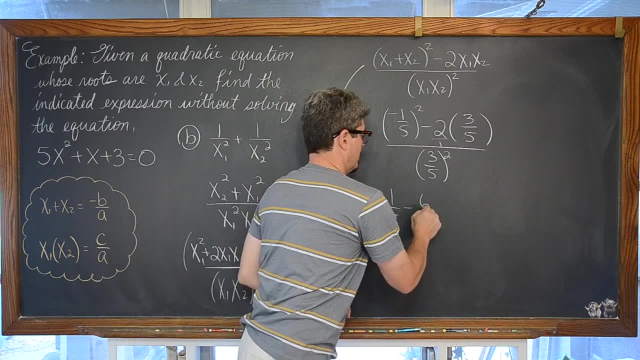 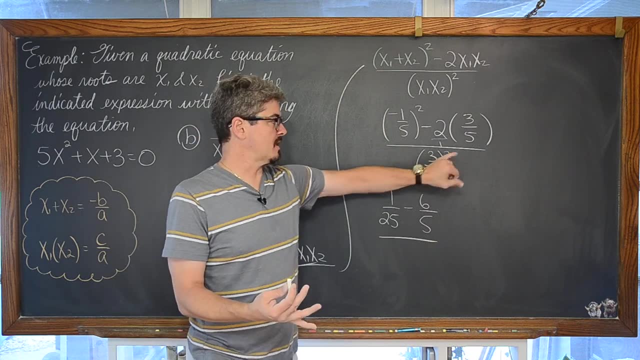 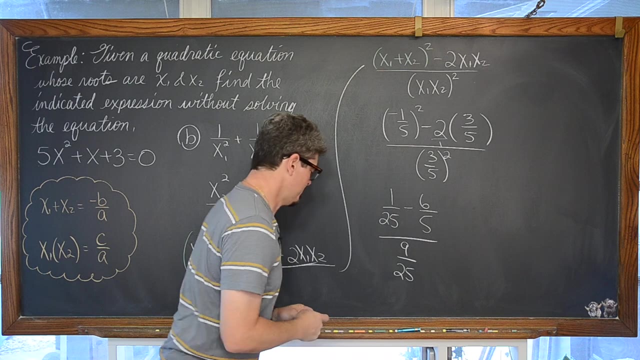 two over one. So two times three is six. 1 times 5 is 5, over you're squaring a fraction. you're squaring both the numerator and denominator separately. so 3 squared is 9,, 5 squared is 25.. We're getting excited. We're almost done. 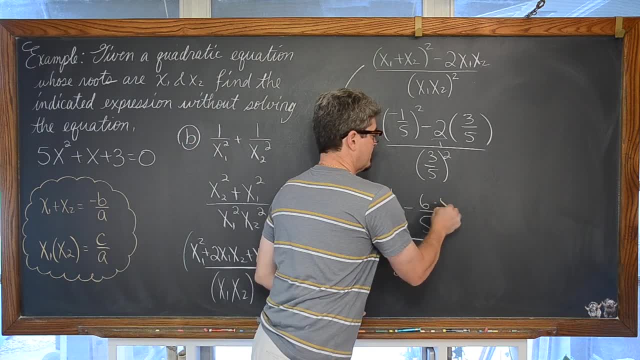 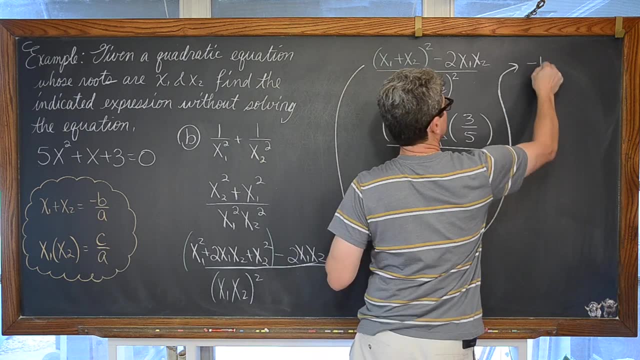 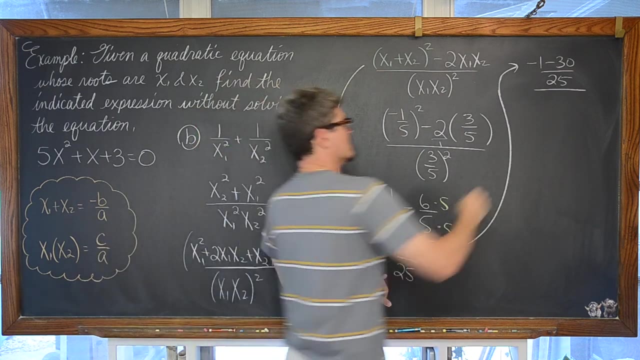 We need a common denominator. so we're going to multiply the numerator and denominator by 5 over here on our second term And we have negative 1 minus 30 over 25, our common denominator. all of that over 9 over 25.. You have since I showed this step very thoroughly. 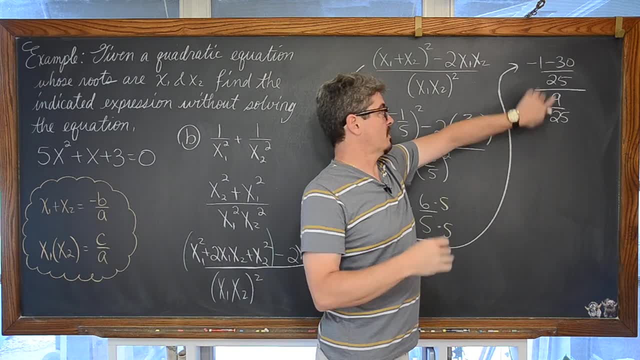 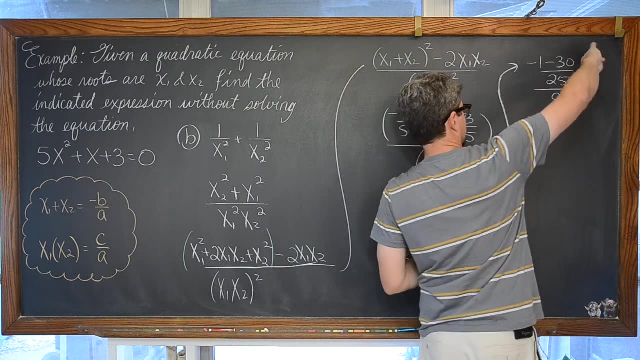 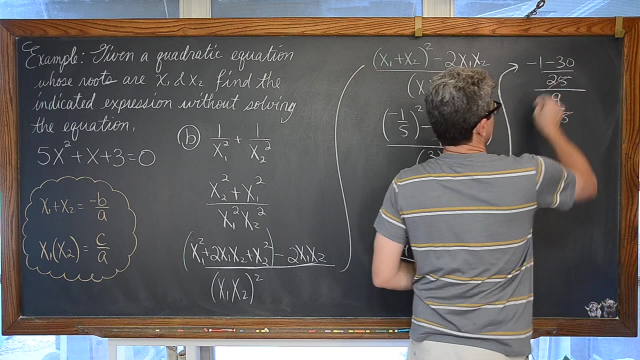 in the last example, our fraction in the numerator and our fraction in the denominator have exactly the same denominator. So when I flip up that at 9 over 25 and make it a multiplication of the reciprocal, make it a multiplication of 25 over 9, these denominators are going to cancel out. So we are looking at whoops. 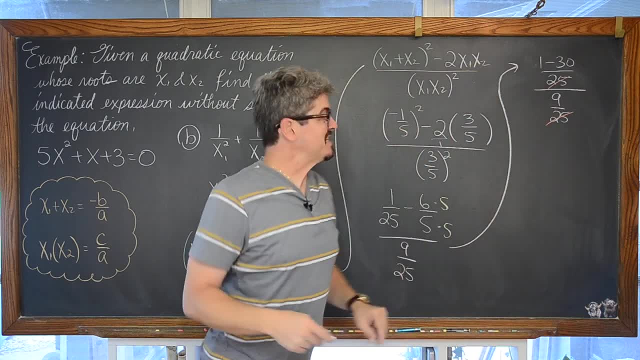 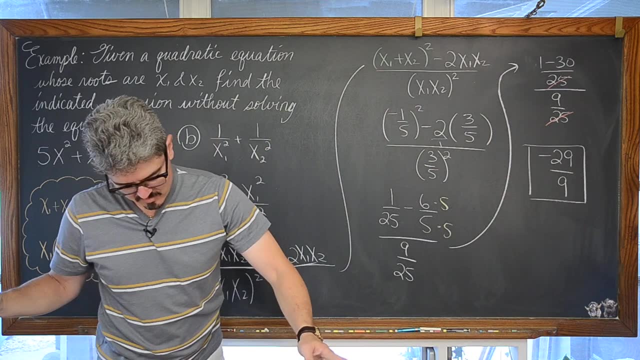 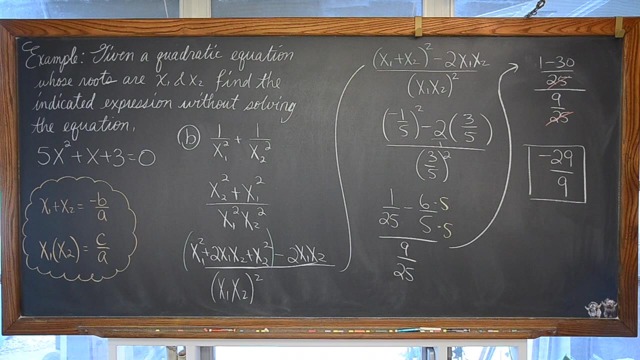 that's a positive one. and I wrote: minus 1 minus 30 is negative: 29 over 9.. And to double check that I have not made an error except for the one that I just caught: boom, That's the end of our second example. Boom, I am in Bam. So we have had a lot of factoring. 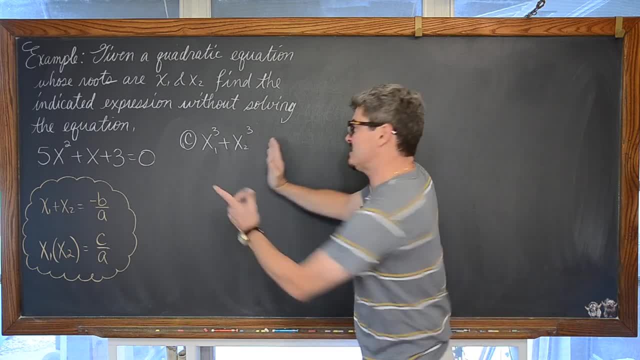 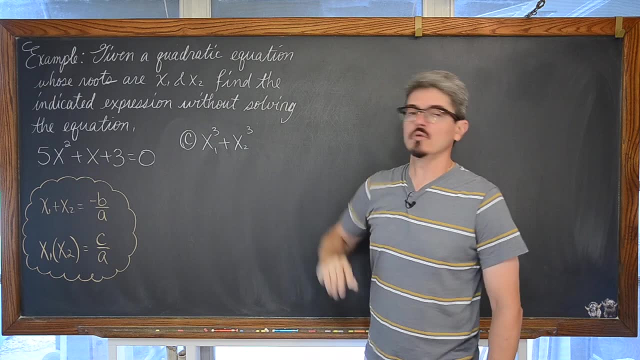 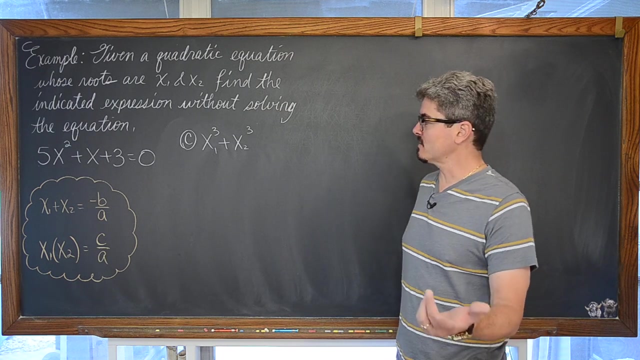 examples in review in this video and we have one more. with our last example, We want to evaluate the sum of x sub 1 cubed plus x sub 2 cubed. Yeah, we want to take the roots from this quadratic cube them, add them together and find an answer without actually solving. 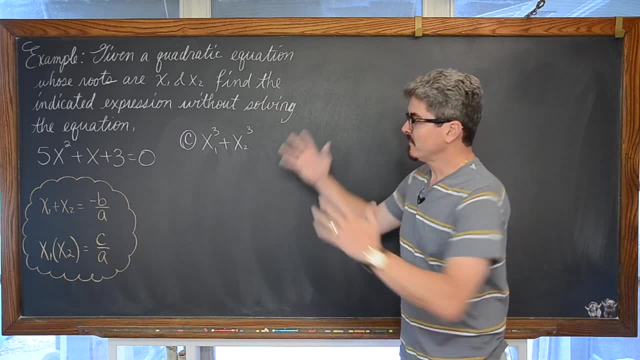 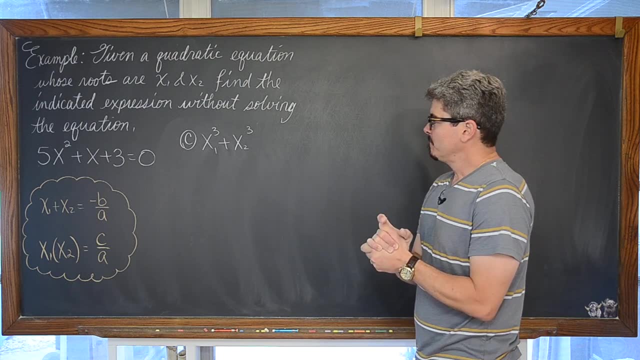 it Using the quadratic. Because what if it was a fifth degree And we were extending this concept onto higher order polynomials? Maybe we wouldn't want to actually have to solve it? Well, you are going to have to remember that again. we don't have any powers. we don't 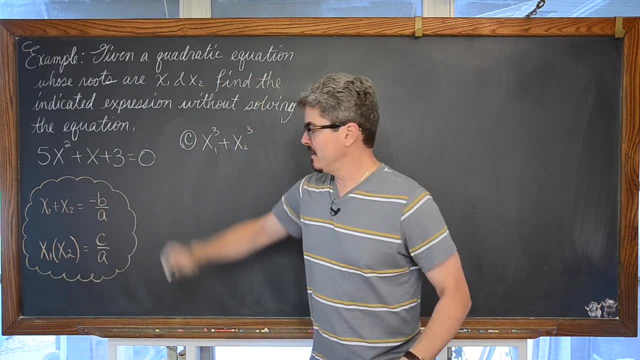 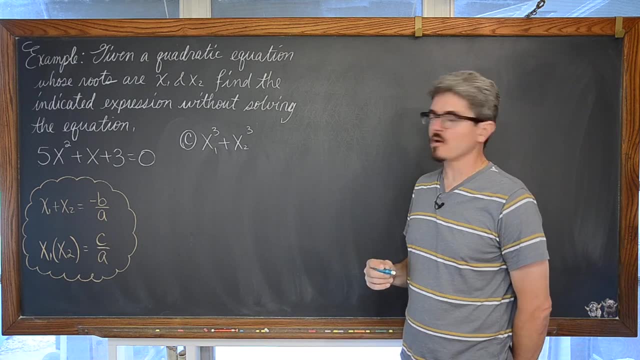 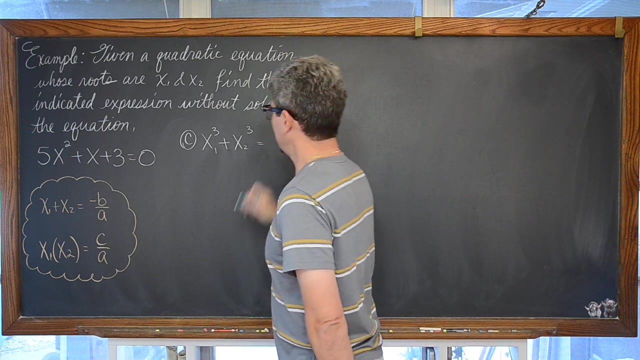 have any subtraction division. it has to look exactly like the sum and the product of these roots to be able to do a straight substitution using the coefficients from our polynomial. That means that we have to factor. We have to factor a sum of cubes And basically this is just a formula. I mean, there is a 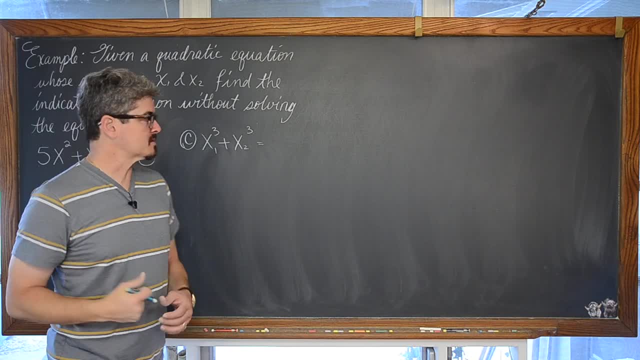 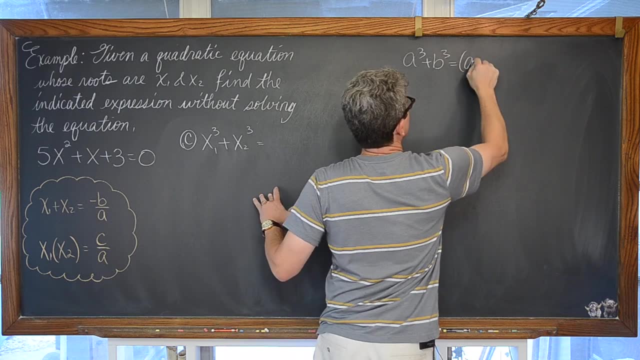 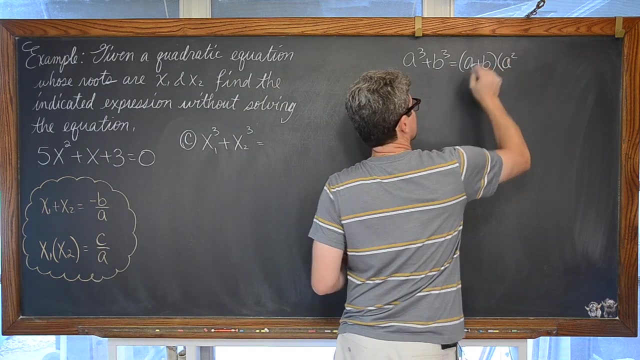 way to prove it or derive it, but we need to be able to pull this out of our tool box and remember that a cubed plus b cubed is equal to a plus b. So you take the cube root of each of those terms and then that is times a squared. Whatever, this is, now you are going. 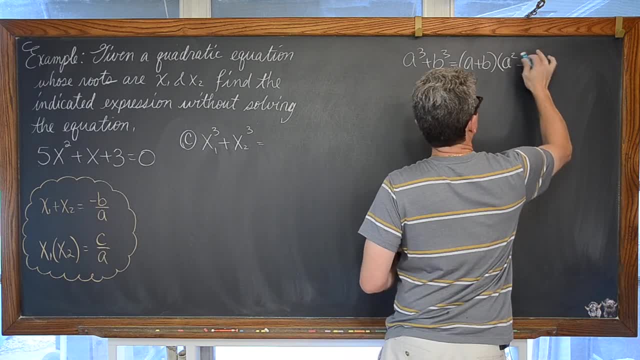 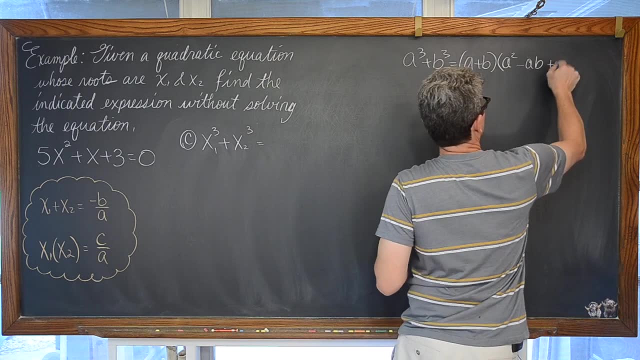 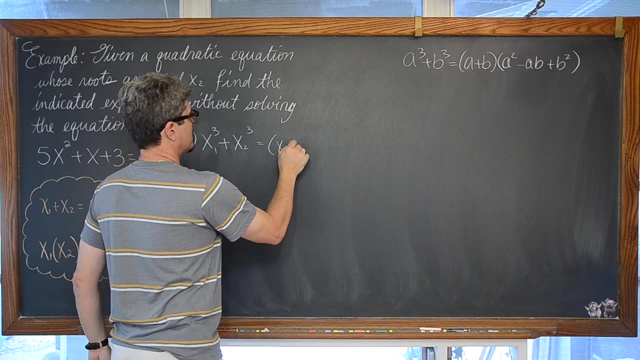 to change the sign. So minus a- b. Every new school year I have to go look up: is that just a coefficient of one there or two? But it is minus a b plus b squared. So this is equal to x sub one plus x sub two. Well, that is nice. We already got a place that we can plug. 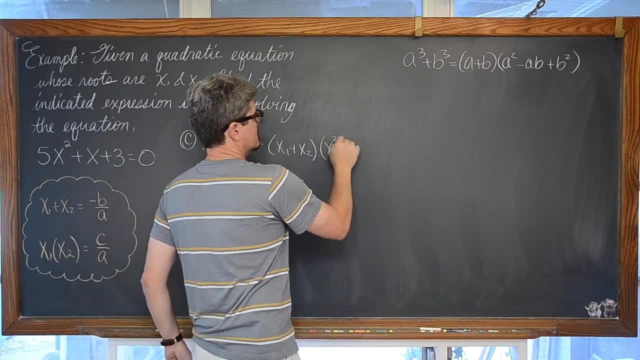 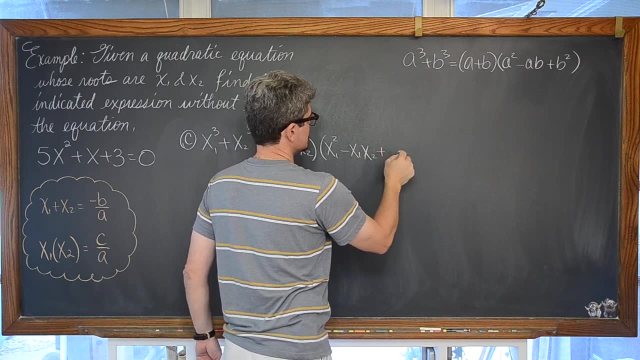 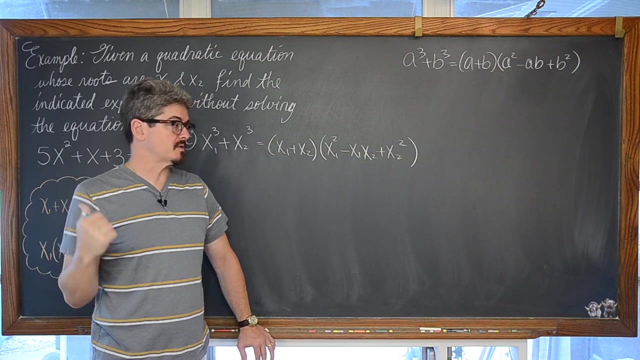 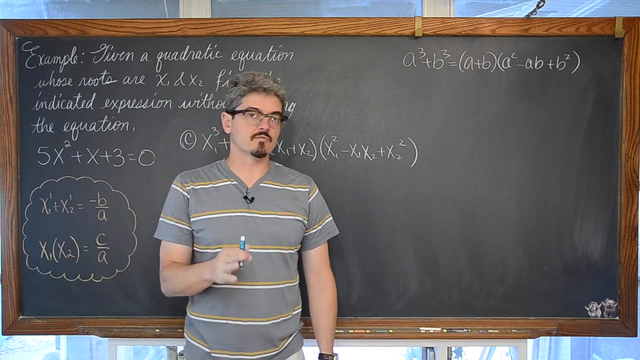 in our negative b over a times x sub one squared, minus x sub one, x sub two, plus x sub two squared. And here we just have the same problem we had in the last example, where we have powers of two on our roots but in terms of sums we have to have powers of one And, like I, 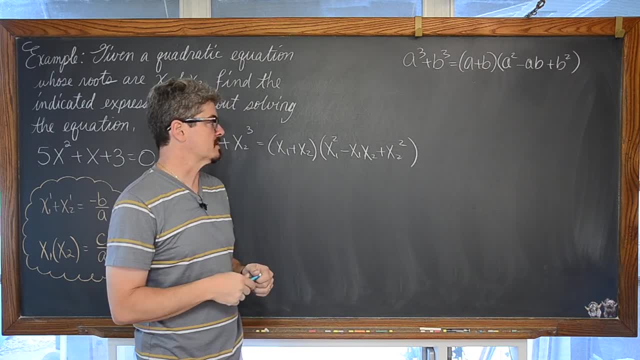 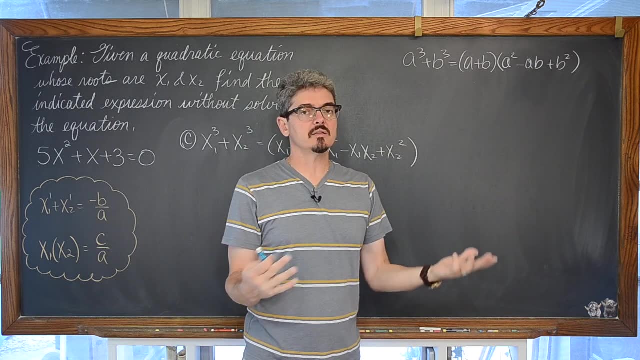 just showed you and kind of a hint as to how to go through this process. I just wrote out with powers of two. I wrote out x sub one plus x sub two to the second power expanded and then saw: okay, well, if I can make my expression look like that, then I can factor it and get. 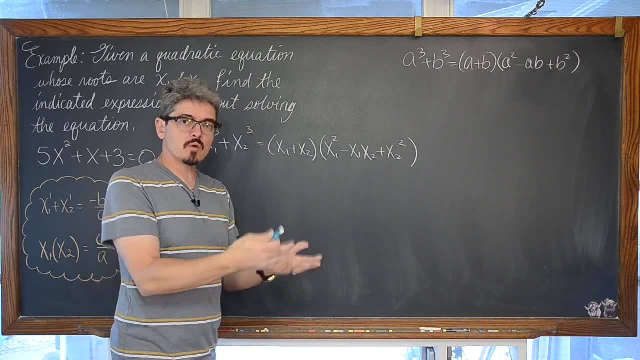 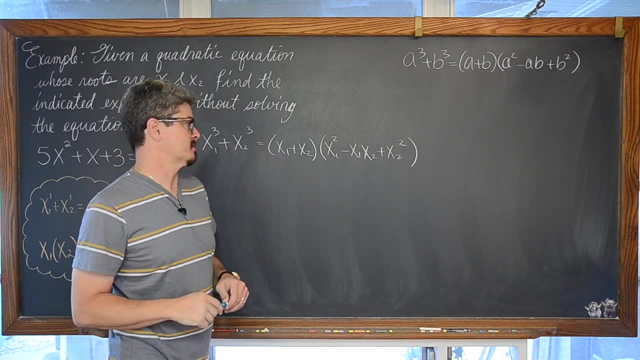 into a form that we can use. Keep that in mind as you do your problems in your book. You might have other versions from other than the three that I am showing you. I need that to be a two x sub one, x sub two, so it factors down to be x sub one plus x sub two squared. So if I am going to make 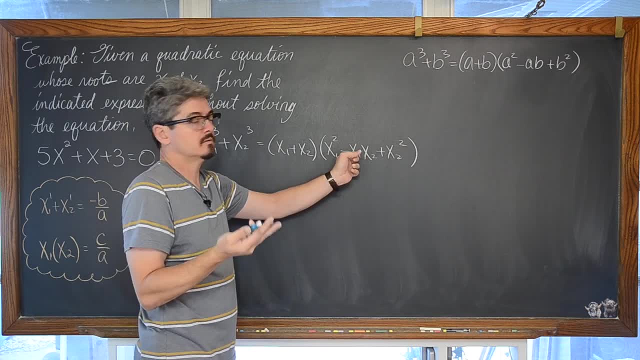 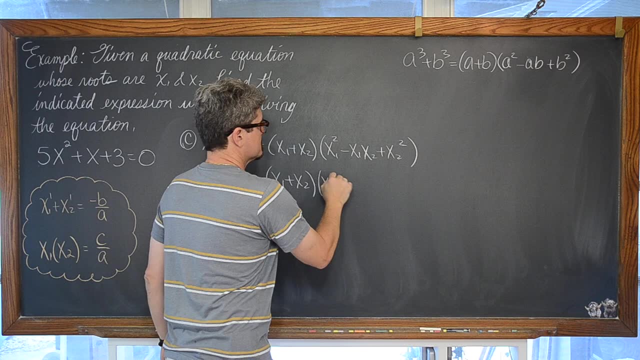 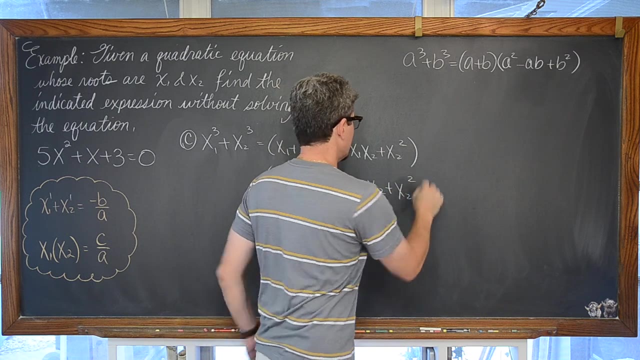 that coefficient go from negative one to two. I need to add three of these terms, So we have x sub one plus x sub two times x sub one squared plus two x sub one plus x sub one plus x sub two squared. But remember I had to add three x sub one, x sub two to 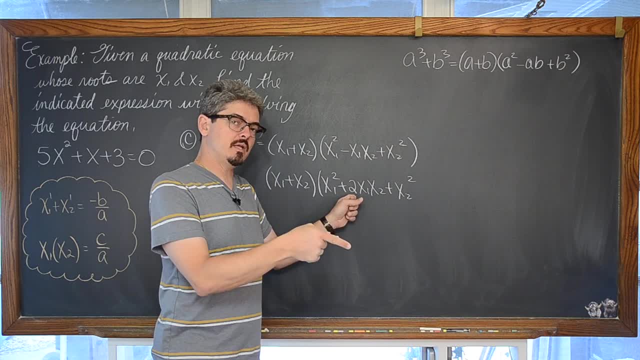 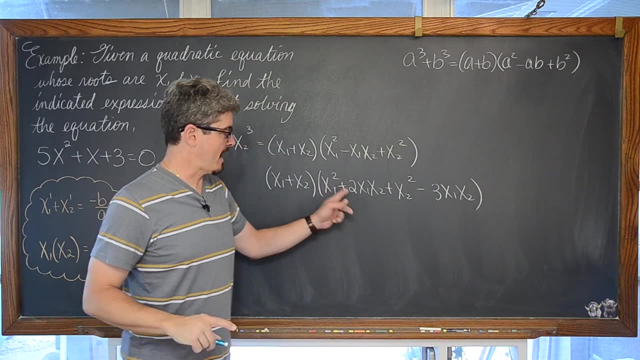 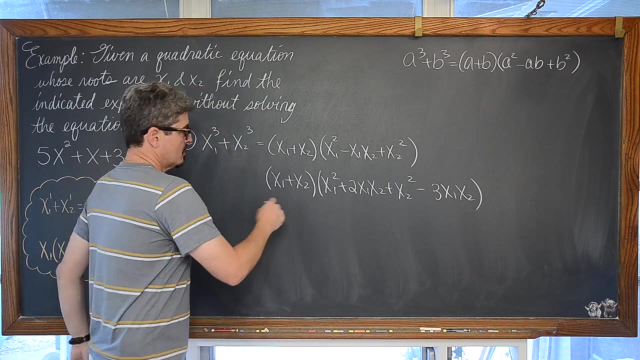 go from negative one to two. So if I am going to add three I have to then subtract three. So minus three x sub one, x sub two. So I added three and subtracted three, which is effectively just adding by zero. So I just made this look different. I didn't change its value. So this: 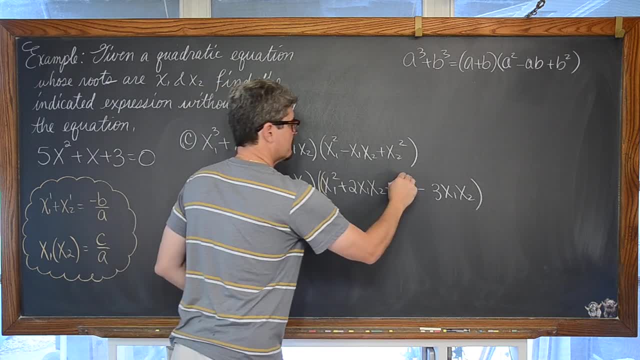 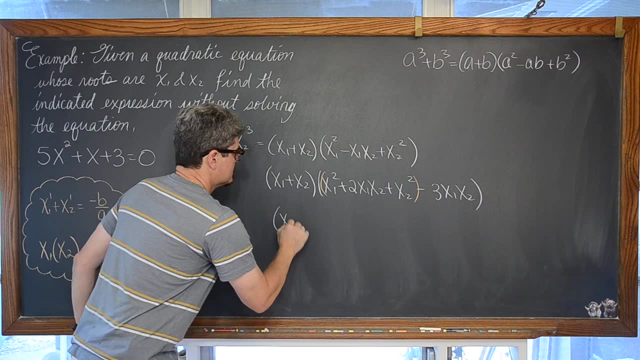 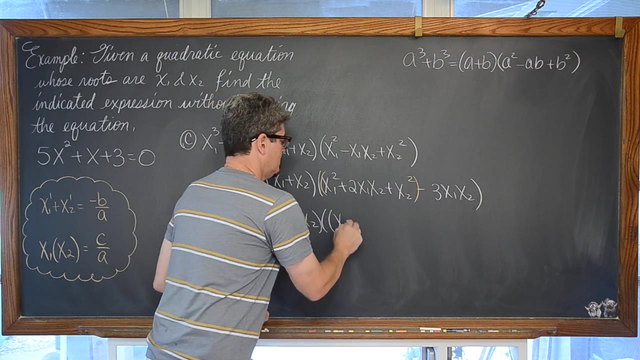 once again, like our previous example, is problem solved. So remember that the term x sub one is a factorable. it's actually a perfect square trinomial. I'm going to get all fancy and use some vocab: x sub 1 plus x sub 2.. Now this is being factored to be x sub 1 plus x sub 2, squared minus 3 times x sub 1. 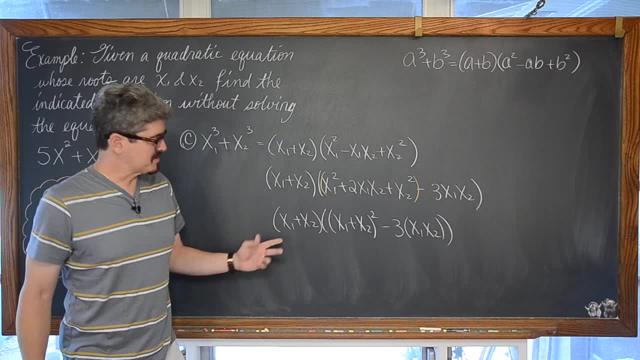 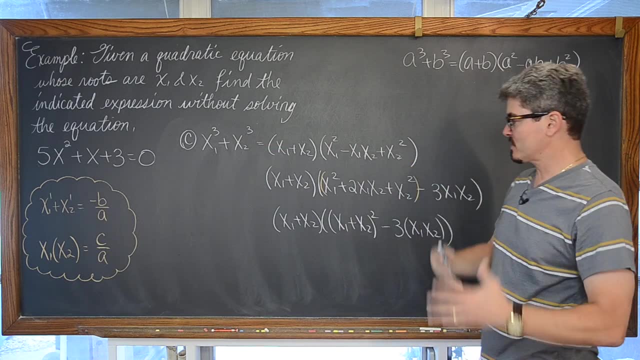 x, sub 2.. Good, Got all my parentheses in the right spot. Sum: sum product of roots. That means we can just go to our quadratic equation, pull out the appropriate coefficients and for the sum, it's negative b over a. it's negative 1 over 5.. 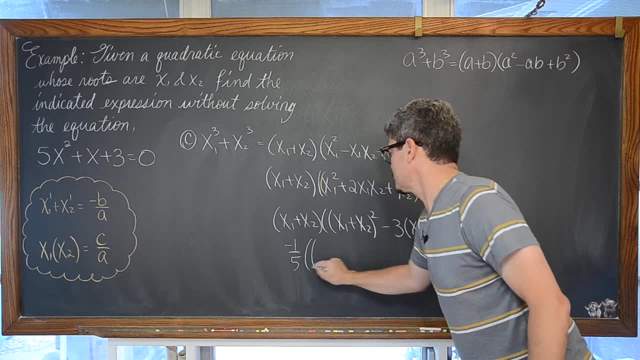 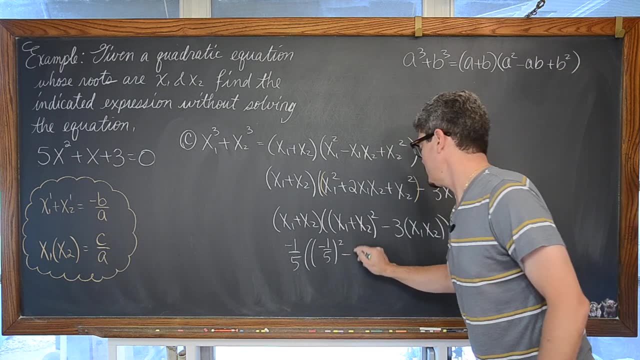 Oh, the air just shut off. That's awesome, And we have another negative 1 over 5.. I do apologize for the hum in the background as I made this video, but it's Florida, it's summer and the air conditioner is right out the window. 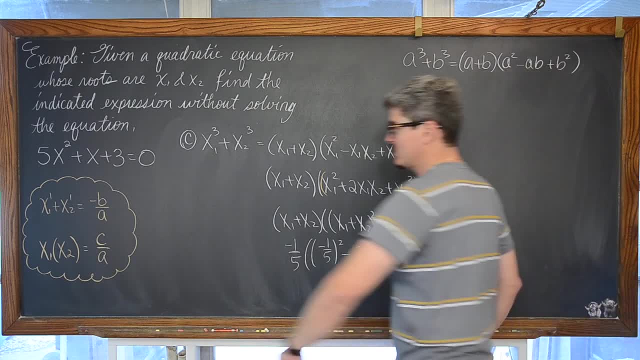 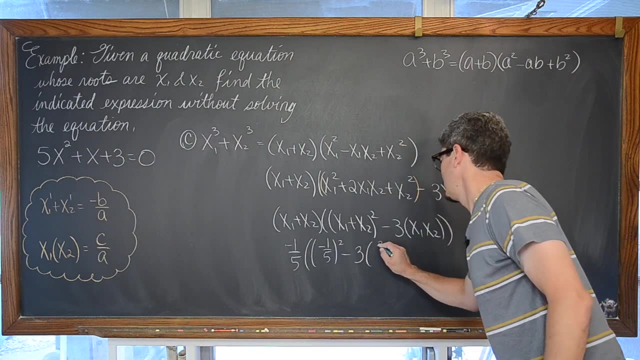 The sum. here we have negative 3 times the, not the sum, but the product. So negative 3 times c over a. Negative 3 times c over a, So 3 fifths. Now, just like before, we basically just have arithmetic to finish this question up.